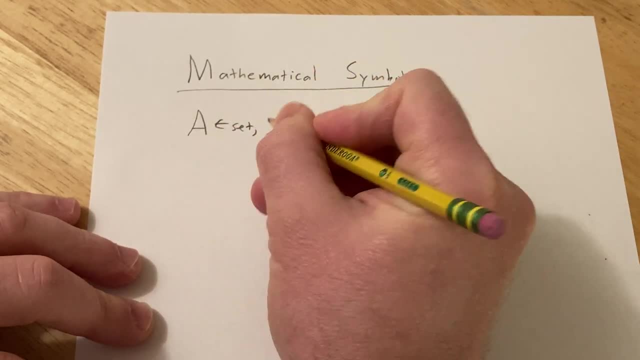 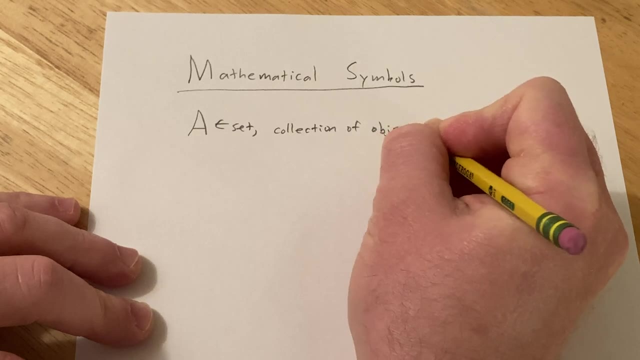 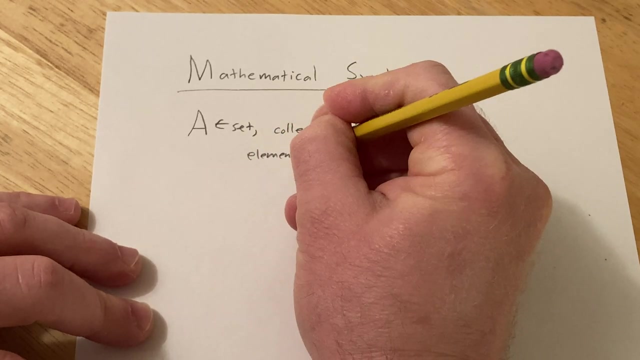 So this is called a set And a set is basically just a collection of objects. So collection of objects, So the things that are in the set, they're called elements of the set. You can also call them members, So those are the things that are inside. 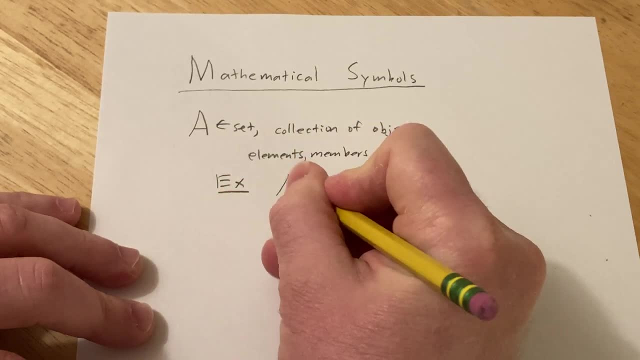 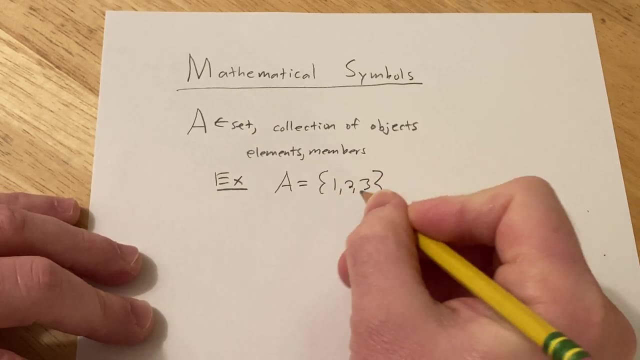 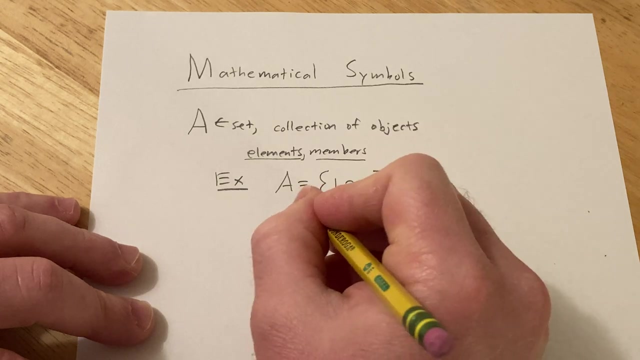 So let's just do a simple example here so you can see: Say we have the set containing numbers, So say one, two, three, So this is a set and it contains three numbers or three elements or three members, All the same thing, And so you need some notation to indicate. 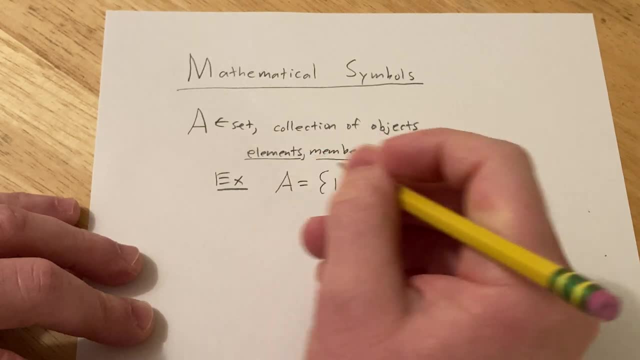 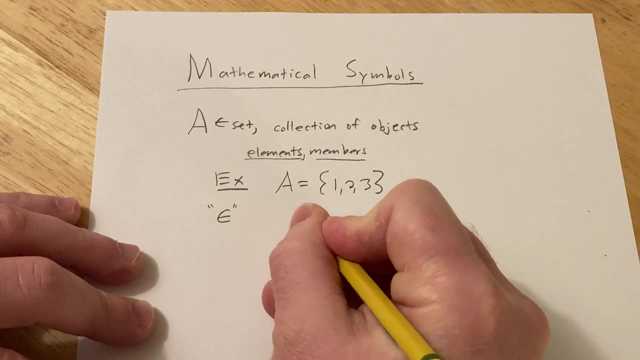 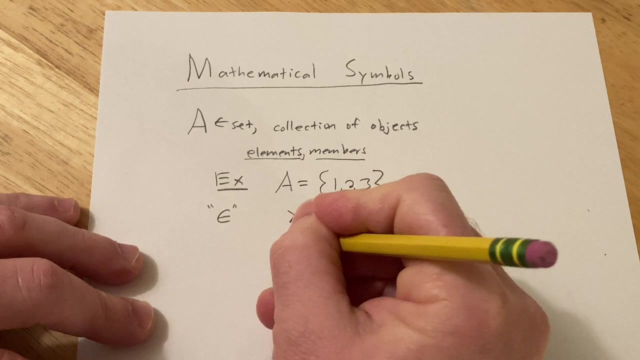 what members are in the set. So what you do is you use this symbol here. Okay, it looks like that, It looks like a little weird symbol, And you say x is an element of A, or x is in A. So that's how you read this. You say is in. 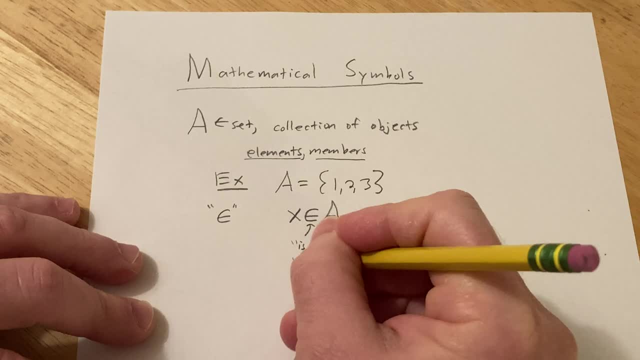 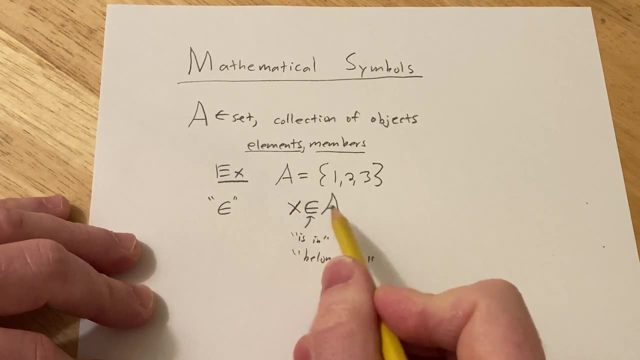 is an element of belongs to. That's another way to say it. So there's various ways to say the same thing. You could say: x belongs to A, x is in A, x is a member of A, x is an element of A Multiple. 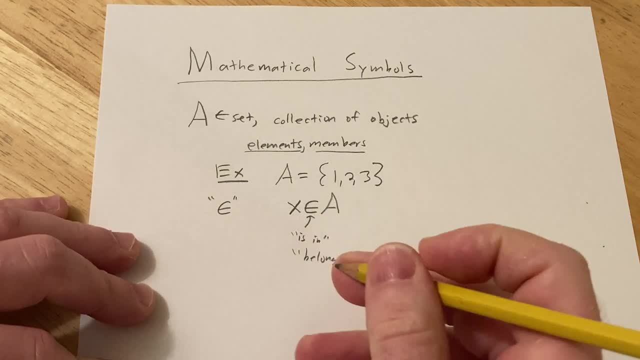 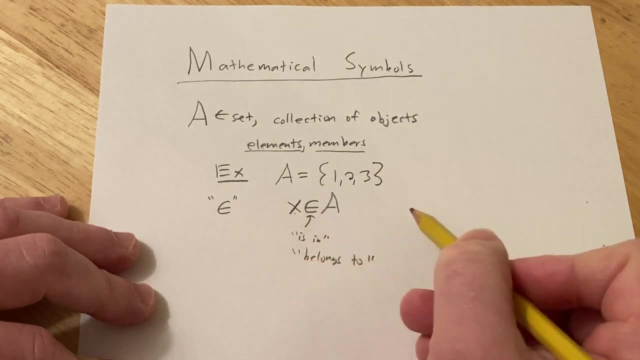 ways to say it And you want to have multiple ways of saying it, so that when you look at this you can just say X is and you pick your choice. personally, I see this and I think X is an A, it's less. 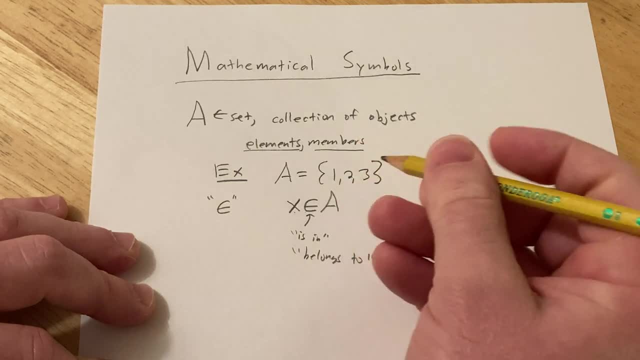 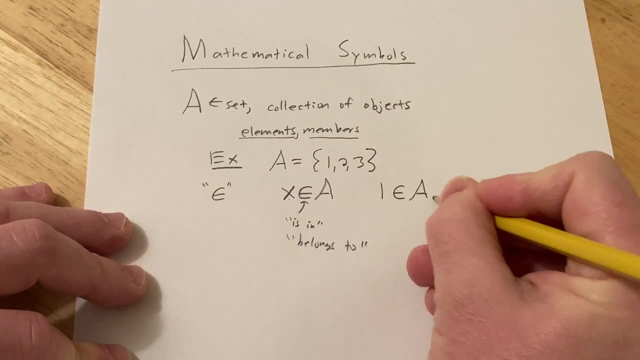 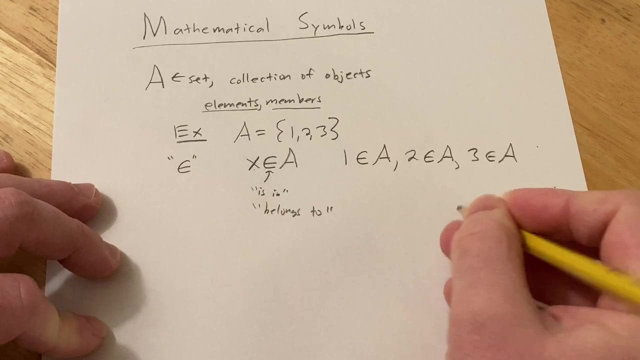 syllables easier for my mind. So, as a concrete example, 1 is an element of the set, so you could say that 1 is an element in A. Likewise, 2 is an element in A. Likewise, 3 is an element in A. What number? 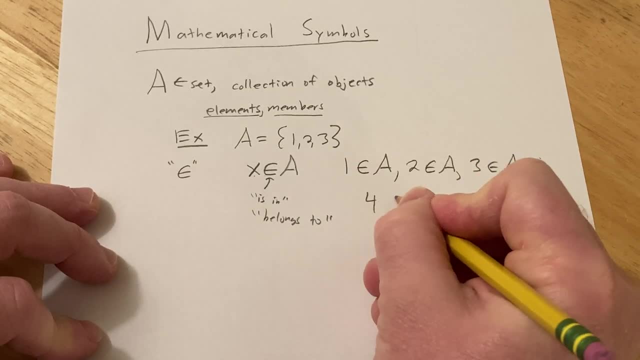 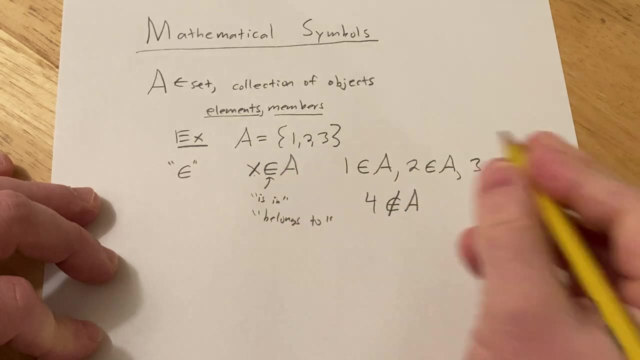 is not in here. Well, 4 is missing. so you could say 4, and then you draw the symbol and you put a line through it and that means 4 is not an element of A, because it's not there. Likewise, the number pi is not an element of A. So now you know a new symbol. it's 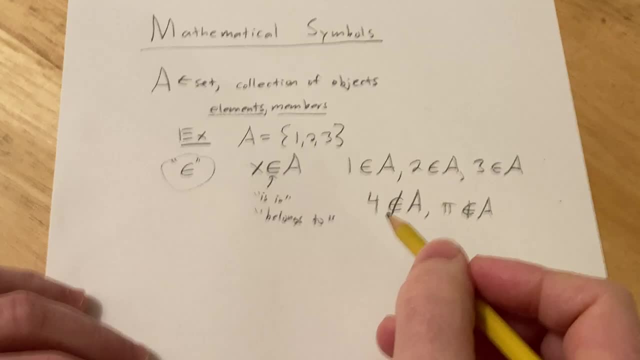 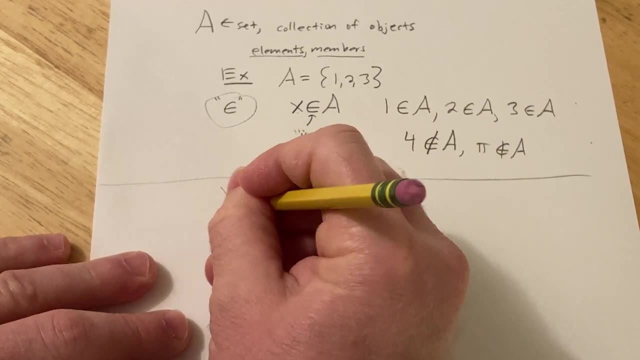 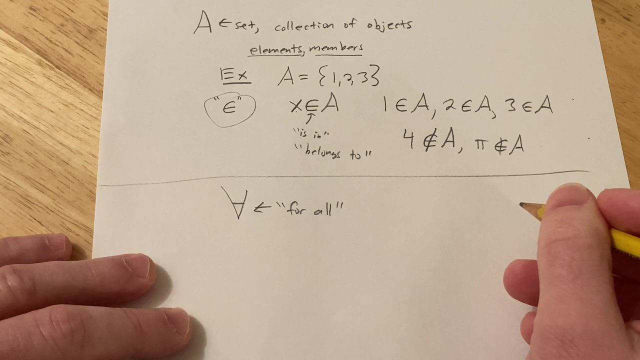 this symbol here and it means: is in, it means belongs to, etc. The next symbol I want to talk about is the for all symbol. So it's like this: upside down A and it means for all, And this is an example of something called a quantifier. okay. 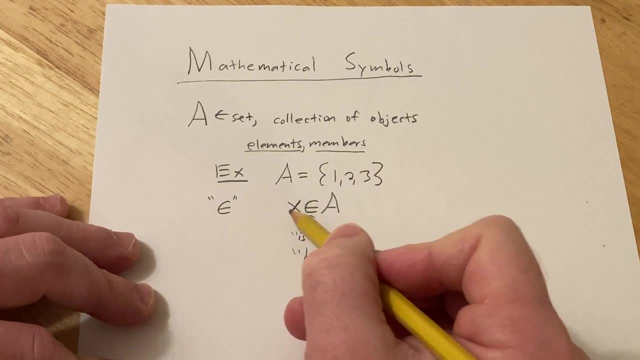 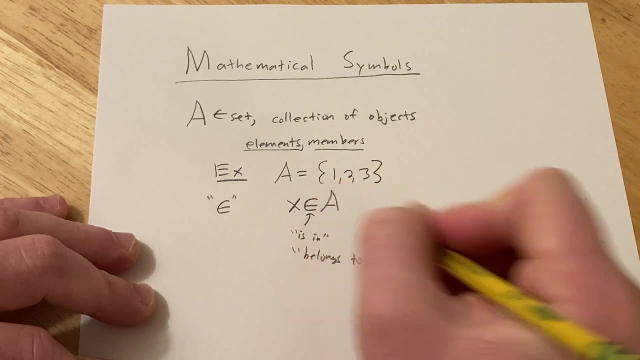 X is and you pick your choice. personally, I see this and I think X is an A. it's less syllables, easier for my mind. So, as a concrete example, 1 is an element of the set, so you could say that 1 is an. 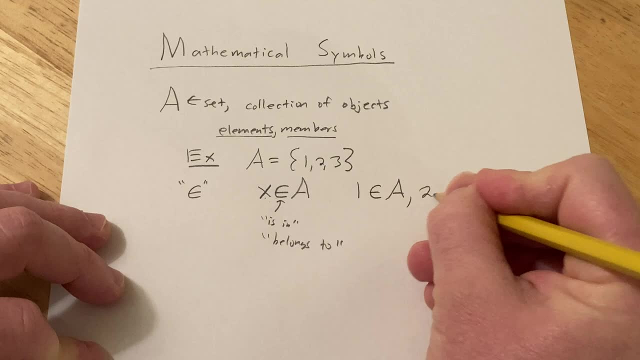 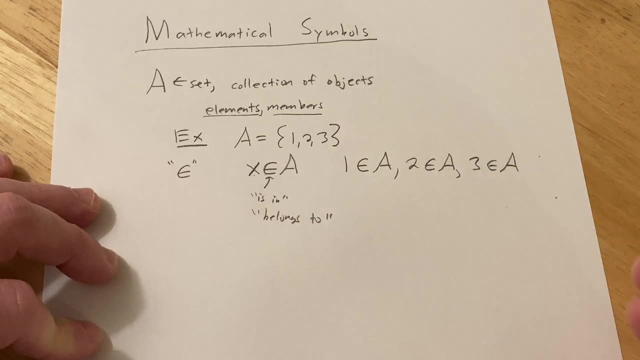 element in A. Likewise 2 is an element in A. Likewise 3 is an element in A. What number is not in here? Well, 4 is missing. so you could say 4, and then you draw the symbol and you put a line. 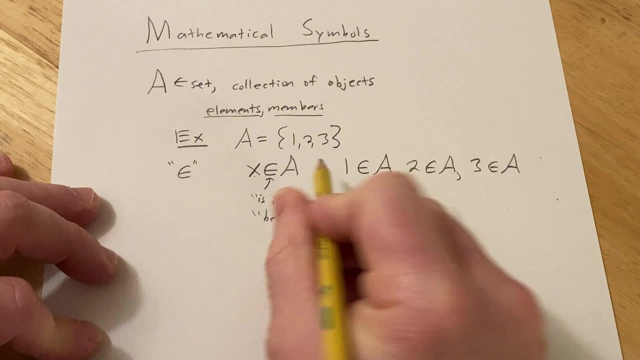 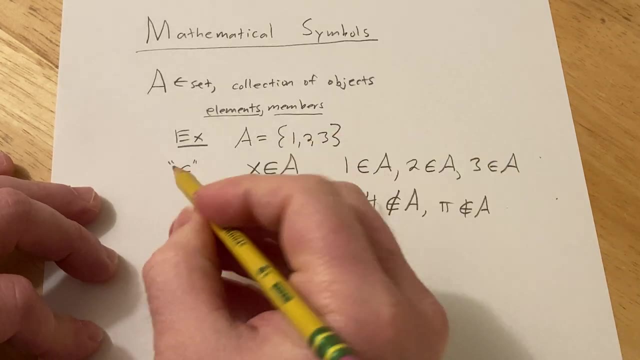 through it. and that means 4 is not an element of A because it's not there. Likewise, the number pi is not an element of A. So now you know a new symbol. it's this symbol here, and it means is in, it means belongs to, etc. 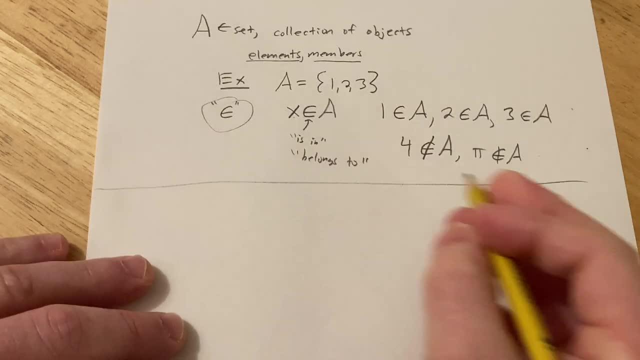 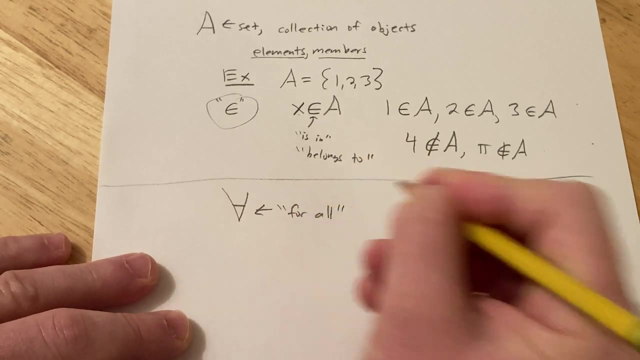 The next symbol I want to talk about is the for all symbol. So it's like this: upside down A and it means for all, And this is an example of something called a quantifier. okay, So it's an example of a quantifier. 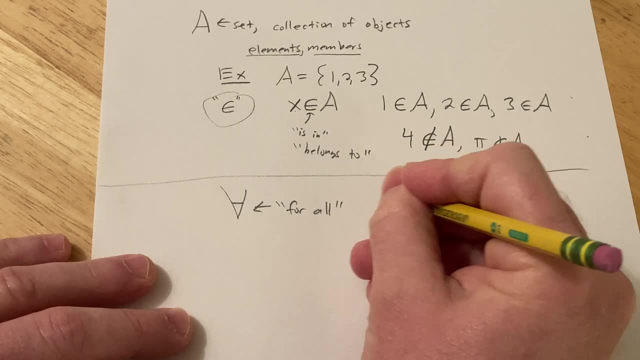 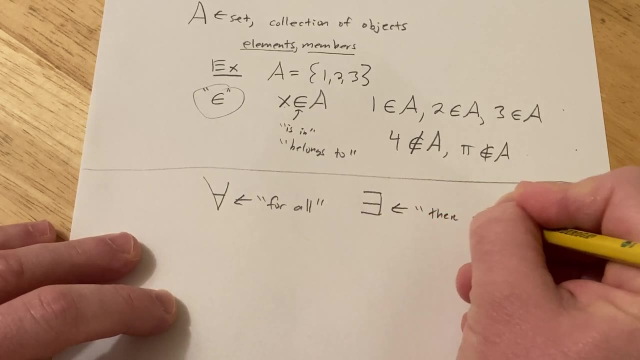 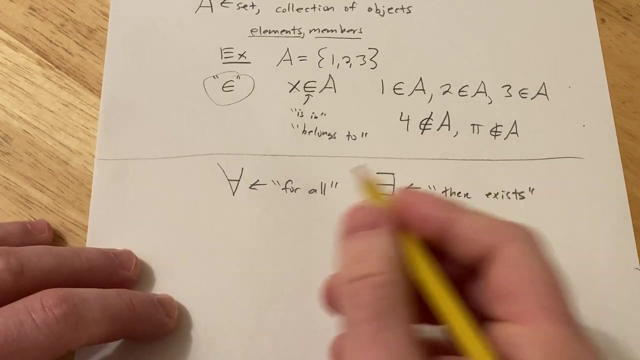 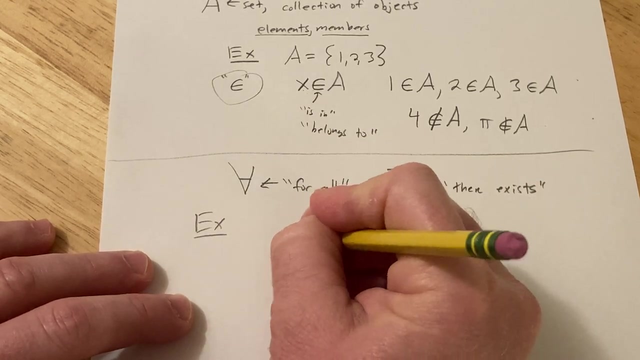 There's other quantifiers. the other one is this one here it's like this: backwards E and this means there exists. okay, So we have for all and there exists. So let's just do some examples. So an easy example would be something like: if you look at X squared, the quantity X squared. 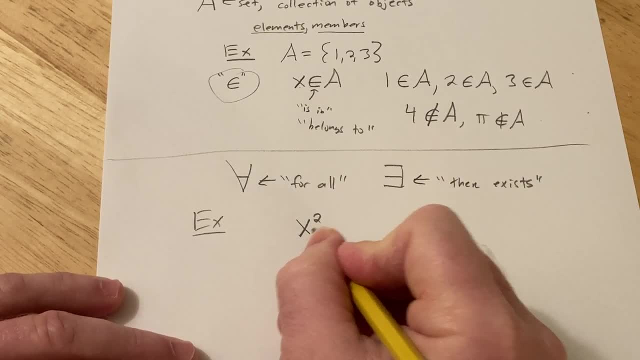 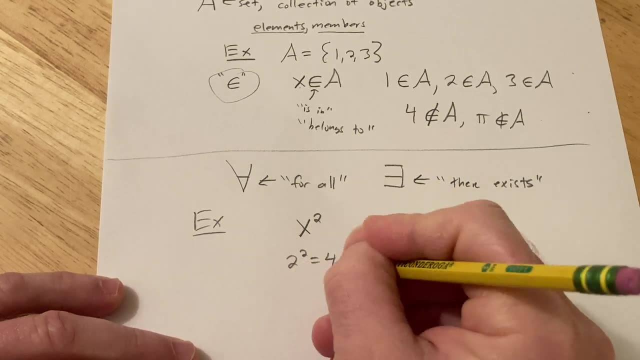 the expression X squared. This is always positive or at zero, as long as the input is a real number. So like, if I plug in 2, I get 4.. If I plug in negative 2, I get 4.. 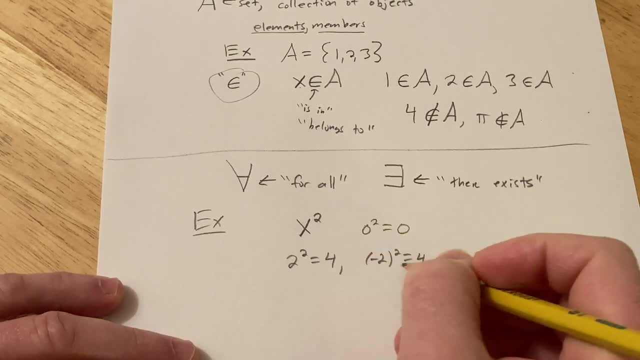 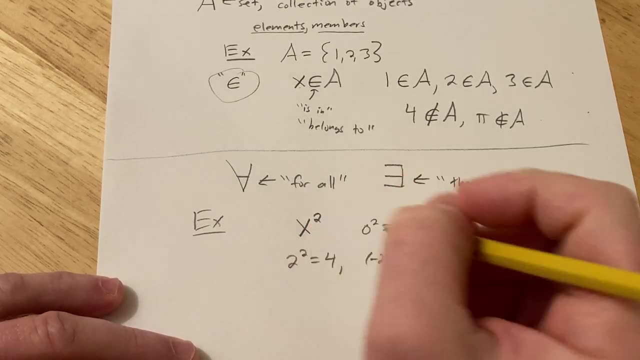 If I plug in 0, I get 0. So as long as you plug in real numbers, right, you don't want to plug in i, because then it might be negative. But if you restrict yourself to real numbers, it's always greater than or equal to zero. 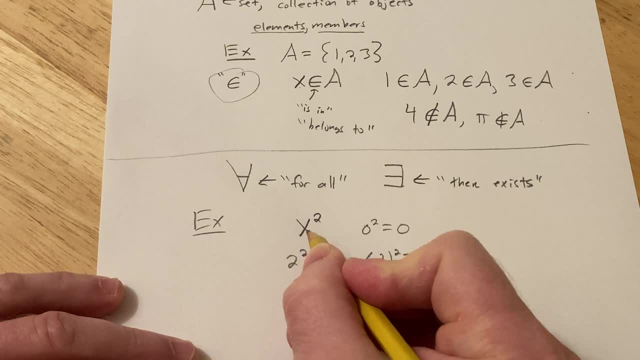 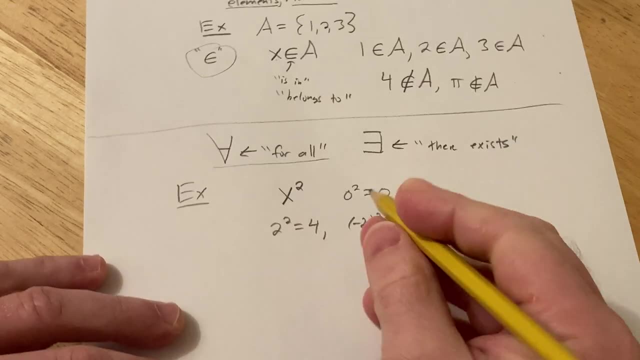 So basically, we want to say that for every real number, this is greater than or equal to zero, for all the real numbers, and that's where a quantifier like this comes in. So in mathematics, the set of real numbers is denoted by this funny R. See how I did. 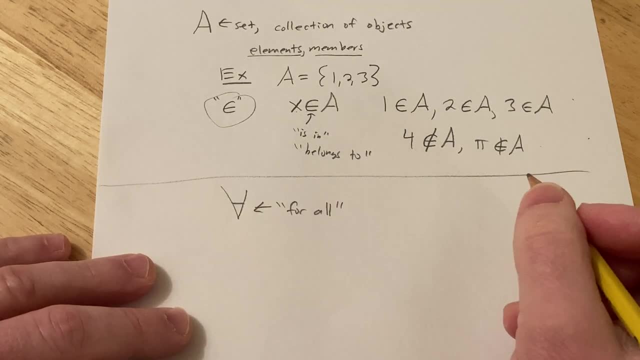 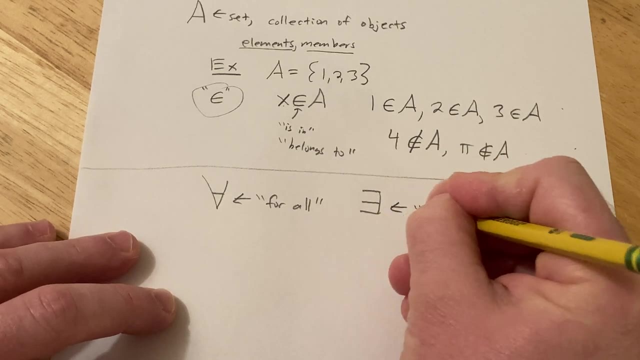 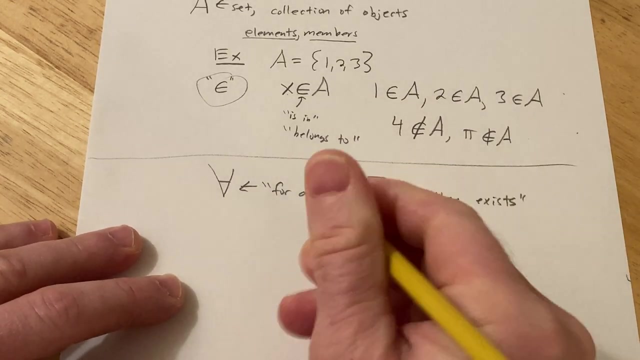 So it's an example of a quantifier. There's other quantifiers. the other one is this one: here it's like this: backwards E and this means there exists. okay, So we have for all and there exists. So let's just do some examples. 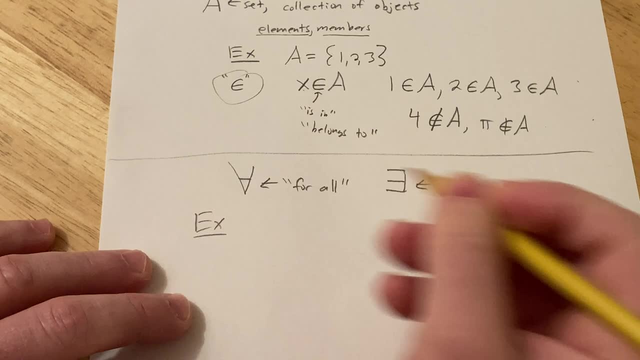 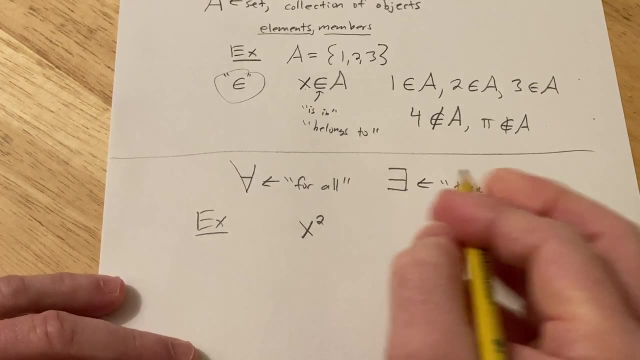 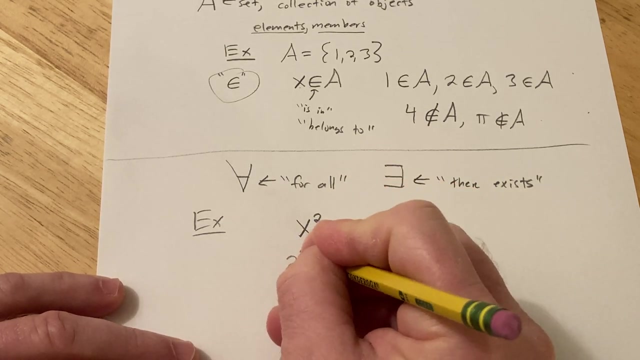 So an easy example would be something like: if you look at X squared, the quantity X squared, the expression X squared, This is always positive or at zero, as long as the input is a real number. So like if I plug in 2, I get 4.. 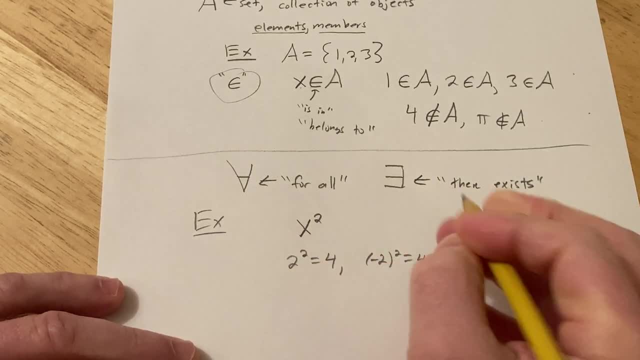 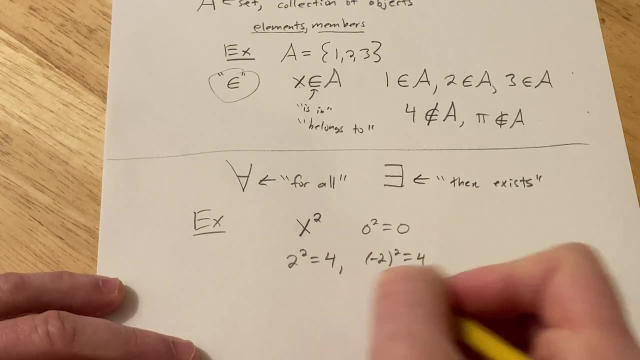 If I plug in negative 2,, I get 4.. If I plug in zero, I get zero. So as long as you plug in real numbers, right, you don't want to plug in i, because then it might be negative. But if you restrict yourself to real numbers, it's always greater than or equal to zero. 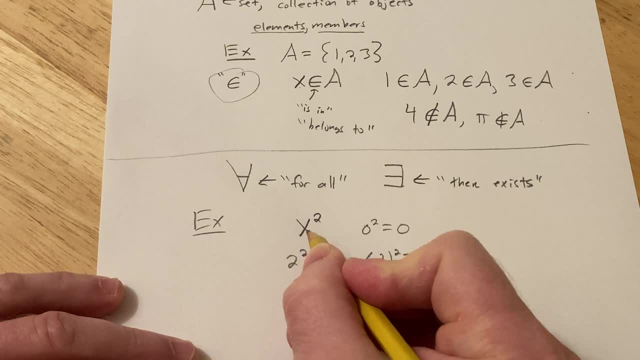 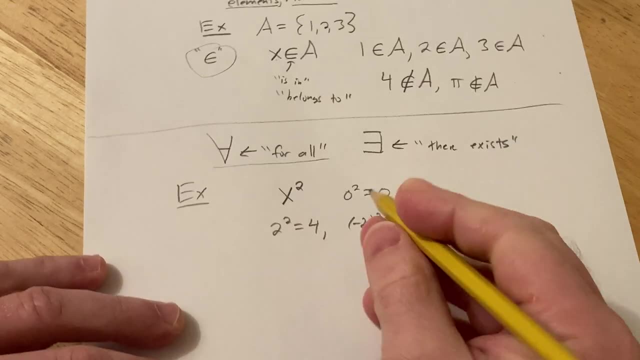 So basically, we want to say that for every real number, this is greater than or equal to zero for all the real numbers, And that's where a quantifier like this comes in. So in mathematics, the set of real numbers is denoted by this funny R. See how I did. 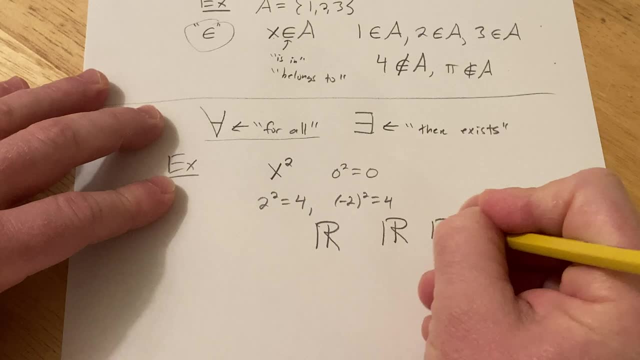 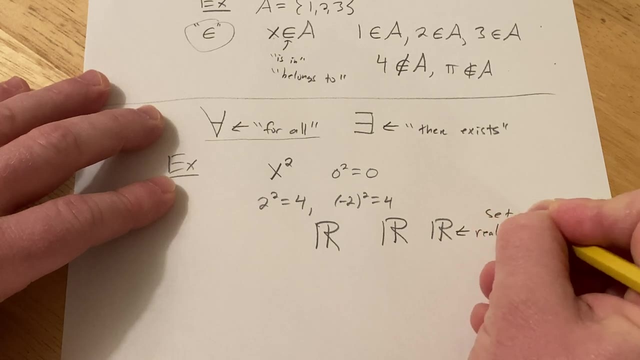 that. Let me do it again: Line line boom, Line line boom. So this is the set of all real numbers. This is the set of real numbers. So if you were to list out this set like this, it'd be impossible, because there'd be too. 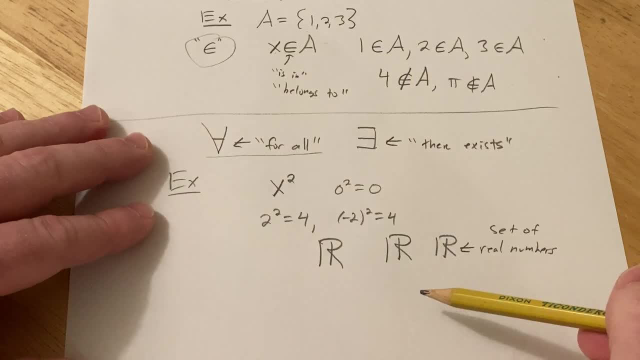 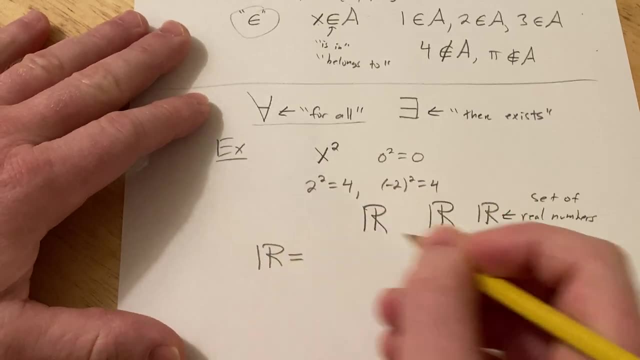 many numbers to list. This is a finite set. You only have three things, But with the real numbers there's infinitely many. A common way that people represent this set in their math classes is using what's called interval notation. So they'll write a parenthesis like this and a negative infinity and they'll put an infinity. 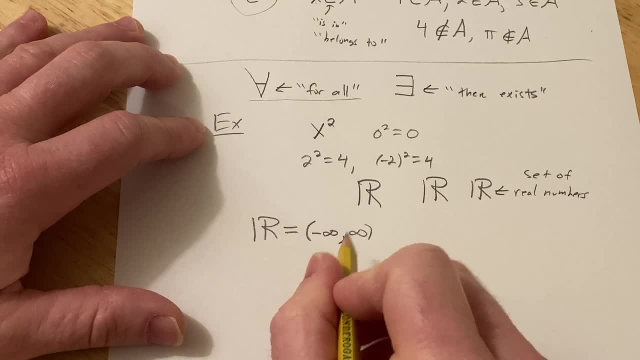 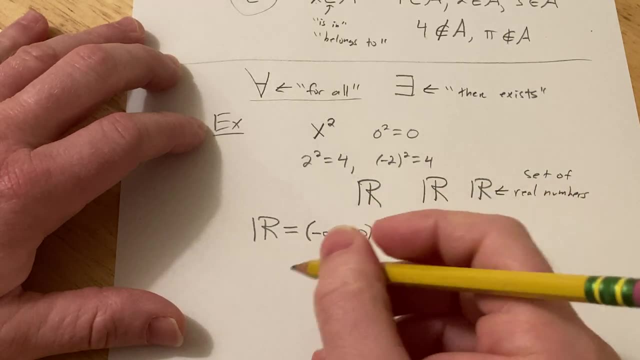 here. Most calculus books use this type of notation, interval notation- because it lends itself really well to the study of calculus. So if you're like in Calc 1, Calc 2, Calc 3, differential equations, even in algebra classes, this is introduced in algebra and that's the notation that most books at colleges. 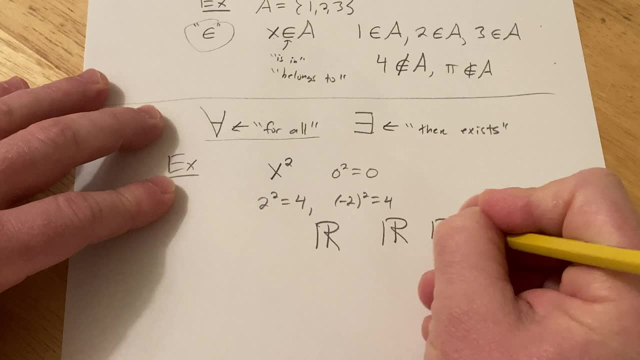 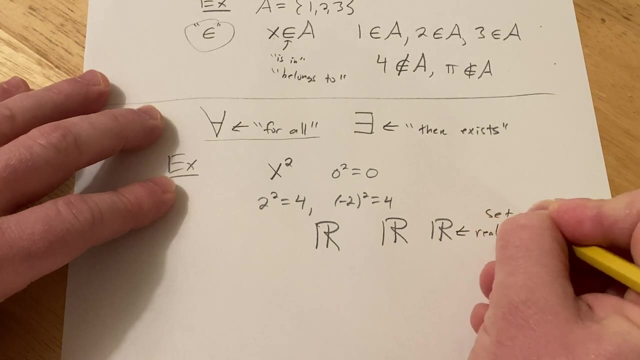 that. Let me do it again: Line line boom, Line line boom. So this is the set of all real numbers. This is the set of real numbers. So if you were to list out this set like this, it'd be impossible, because there would be. 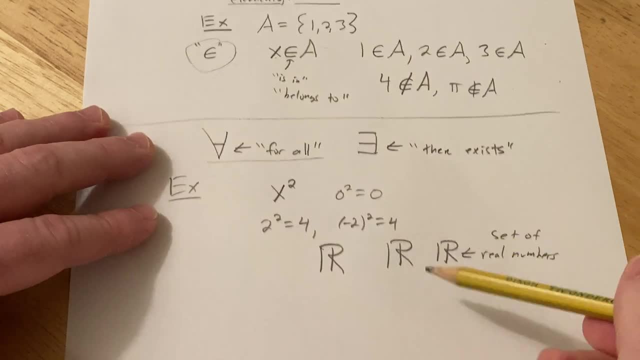 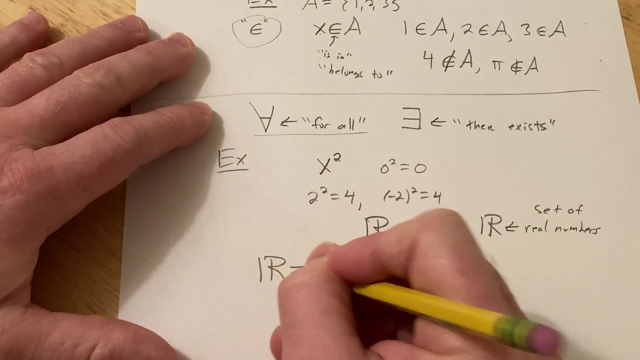 too many numbers to list. This is a finite set. You only have three things, But with the real numbers there's infinitely many. A common way that people represent this set in their math classes is using what's called interval notation. So they'll write a parentheses like this and a negative infinity and they'll put an. 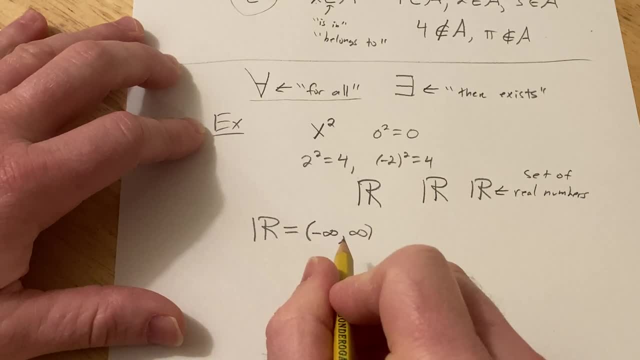 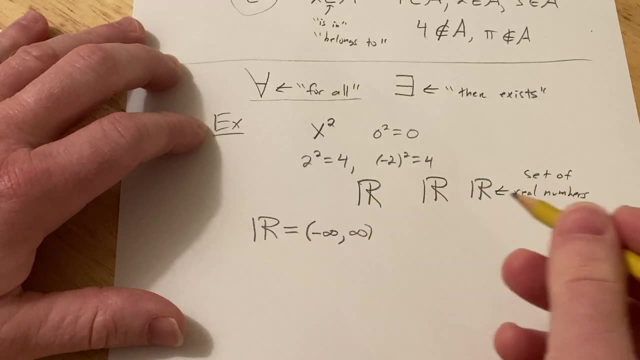 infinity here. Most calculus books use this type of notation, interval notation, because it lends itself really well to the study of calculus. So if you're like in Calc 1, Calc 2, Calc 3, differential equations even in algebra, 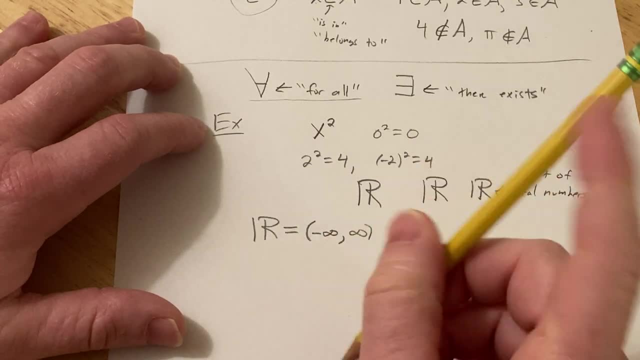 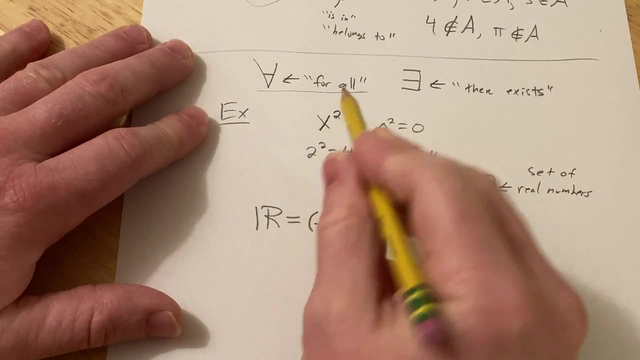 classes. this is introduced in algebra and that's the notation that most books at colleges use. But you have other notation you can use: like this and like this. So now let's try to use the for all symbol to indicate that this is positive or zero. 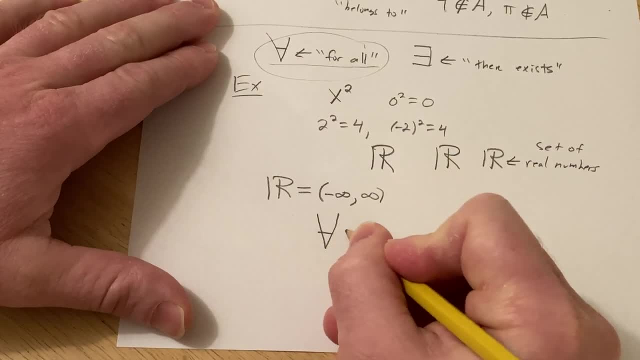 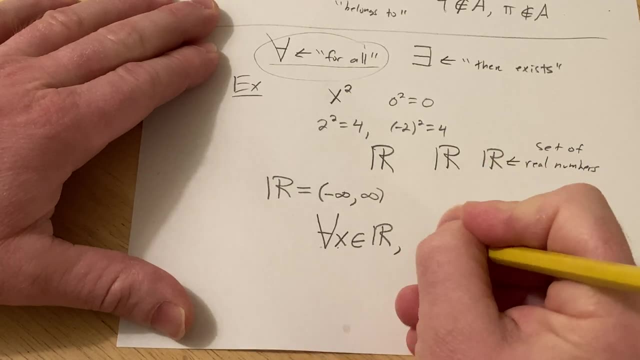 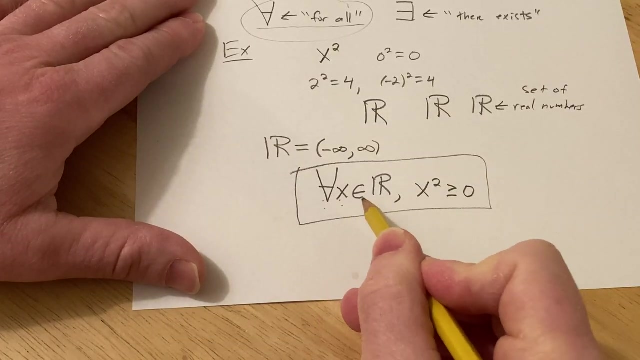 for all x. So you would say for all x in the set of real numbers. I'll put a comma. here We have that x squared is greater than or equal to zero. So that is a true statement, right? So for every x in a set of real numbers. 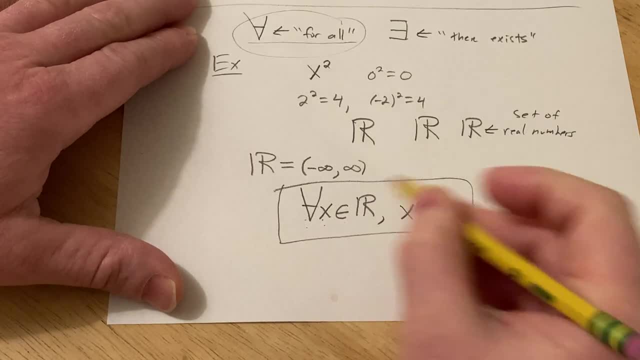 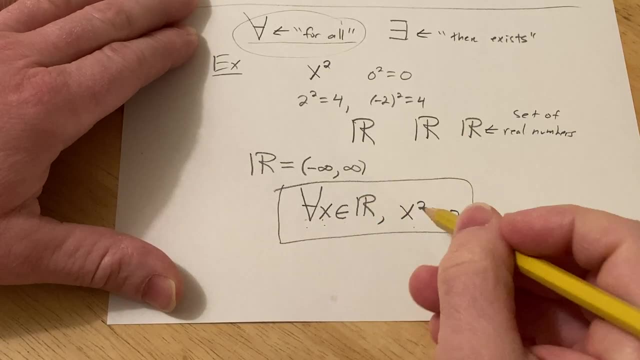 x squared is greater than or equal to zero. So that would be a way of using the for all symbol right. So for all x. in the set of real numbers, x squared is greater than or equal to zero. So that's for all. 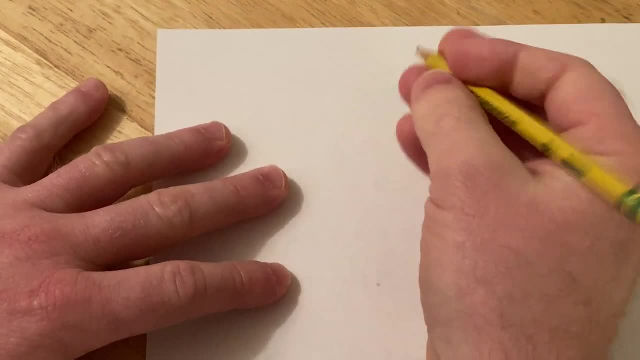 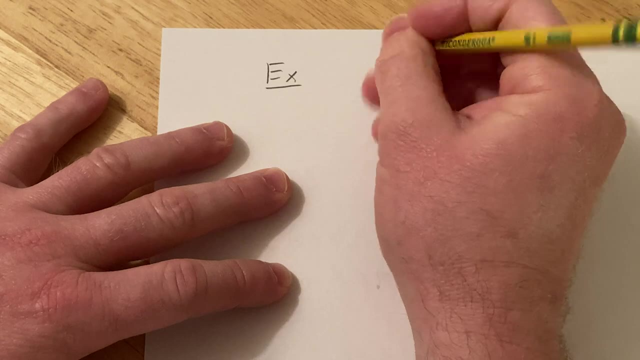 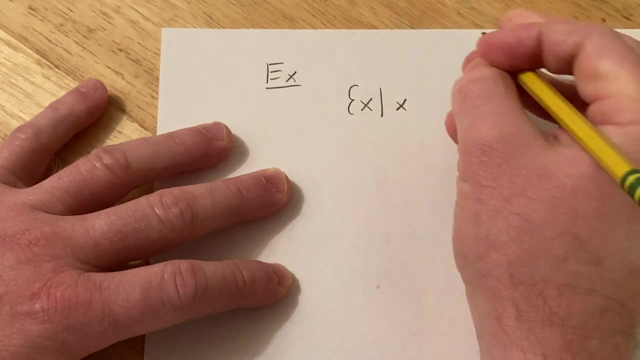 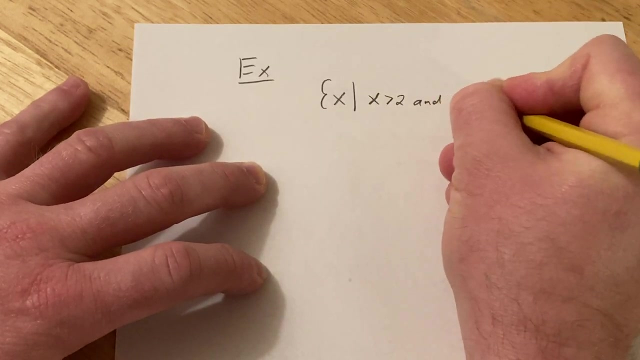 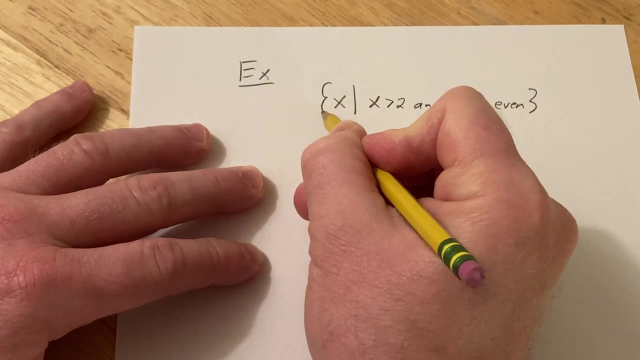 Let's do an example of. there exists. So, for example, let's take the set- This is a simple example- The set x. So this is a set. The way you read this is the set of all x, such that x is greater than 2 and x is even. 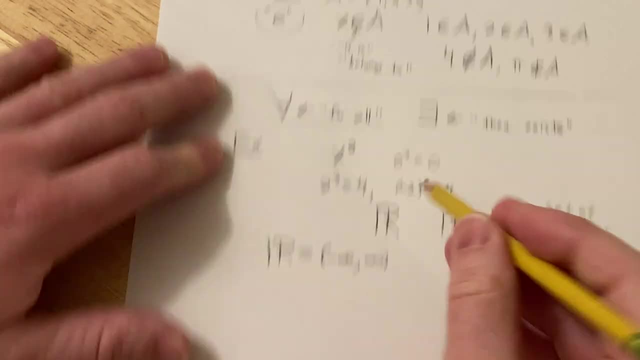 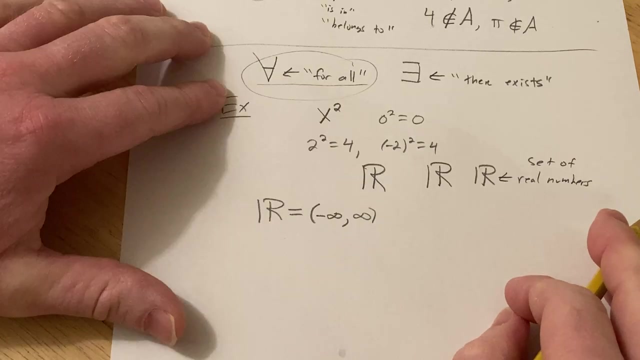 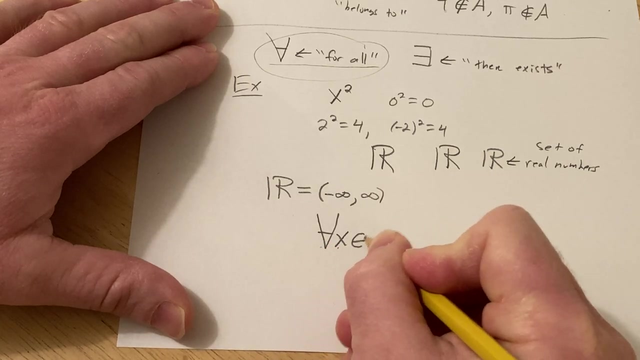 use. But you have other notation you can use like this and like this. So now let's try to use the for all symbol to indicate that this is positive or zero for all x. So you would say for all x in the set of real numbers. I'll put a comma here. we have that. 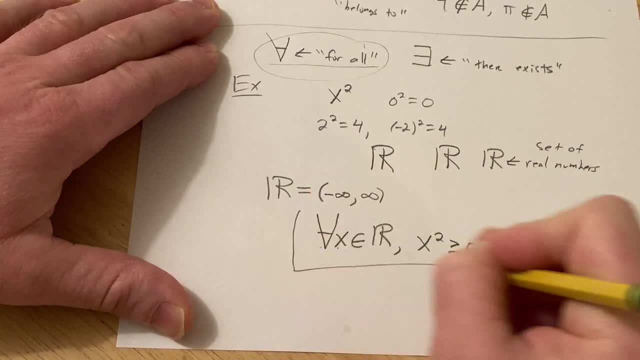 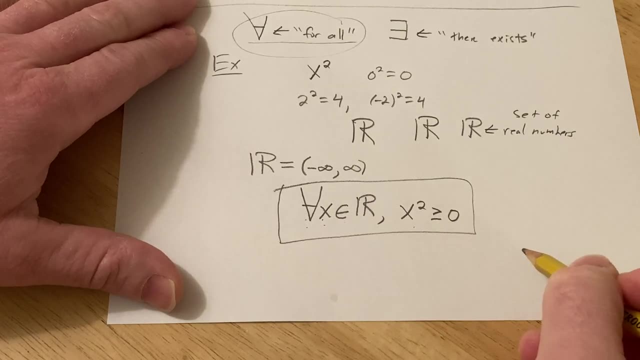 x squared is greater than or equal to zero. So that is a true statement, right? So for every x in a set of real numbers, x squared is greater than or equal to zero. So that would be a way of using the for all symbol, right. 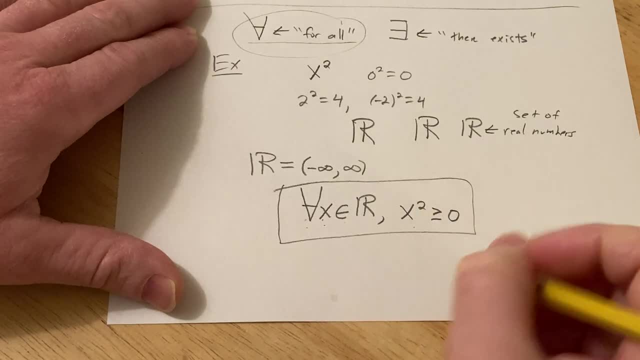 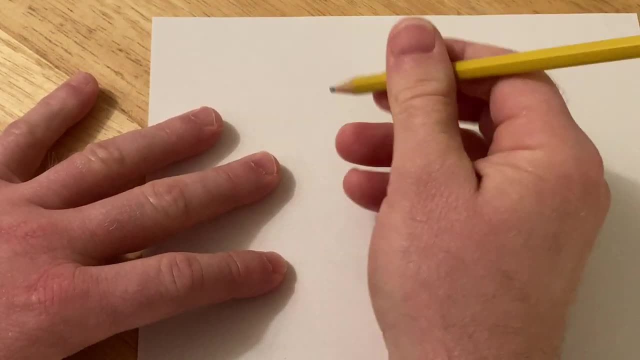 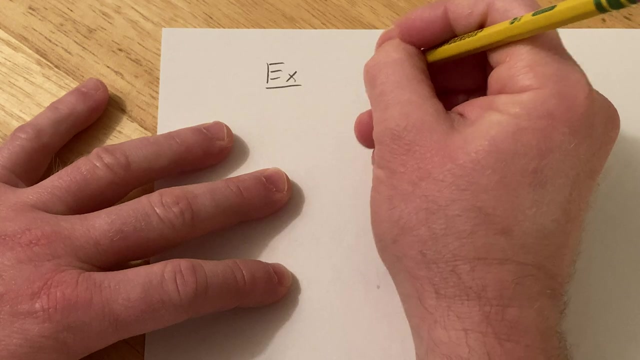 So for all x in the set of real numbers, x squared is greater than or equal to zero. So that's for all. Let's do an example of. there exists. So, for example, let's take the set. This is a simple example. 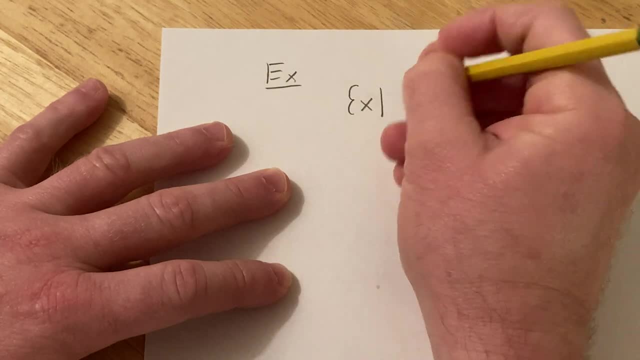 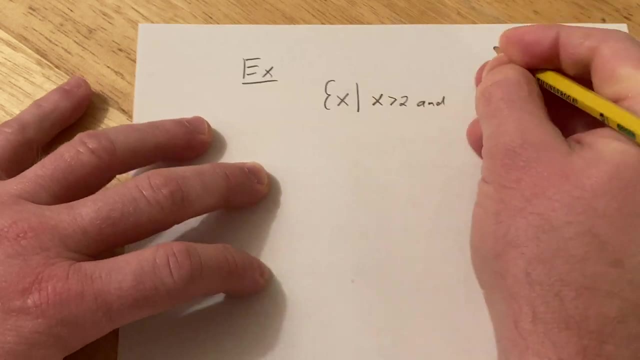 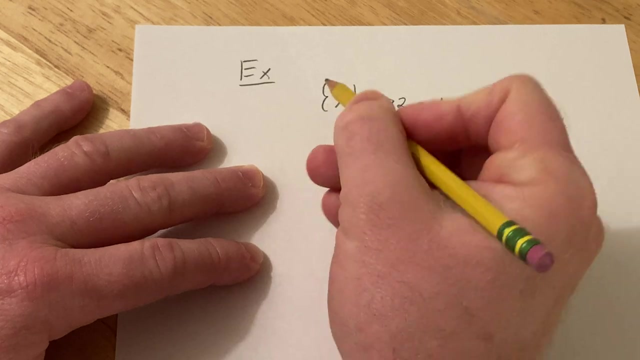 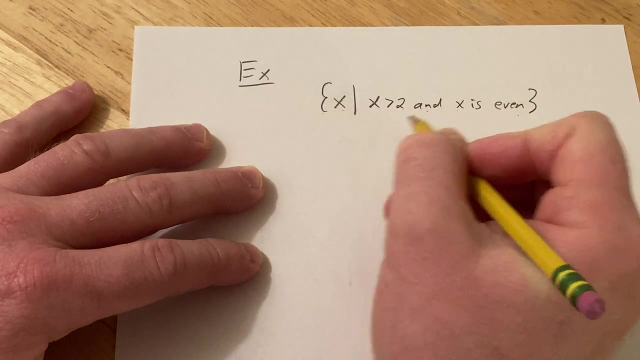 The set x, Such that x is greater than 2 and x is even So. this is the set. The way you read this, is the set of all x, such that x is greater than 2 and x is even So. this set has a bunch of numbers in it. 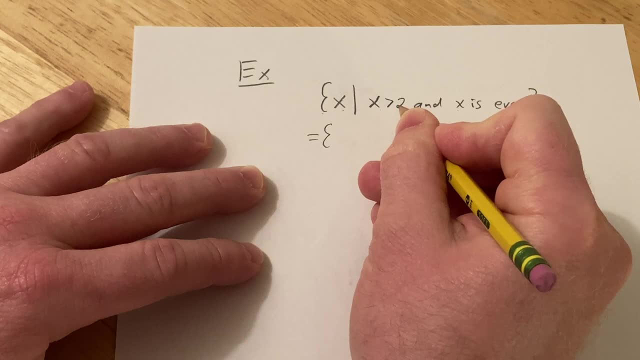 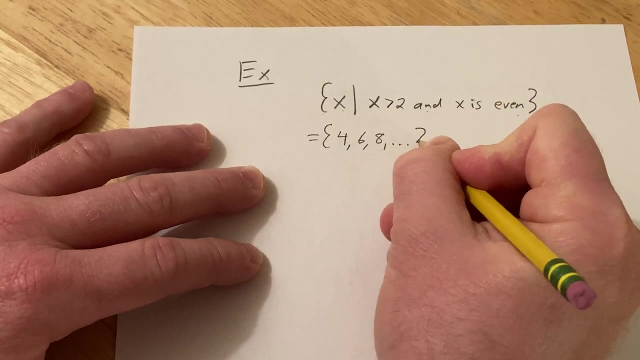 For example, This: The first number that's bigger than 2 and is even is 4.. The next one would be 6,, the next one would be 8, etc. So what we can say about this set is that there are numbers in this set that are divisible. 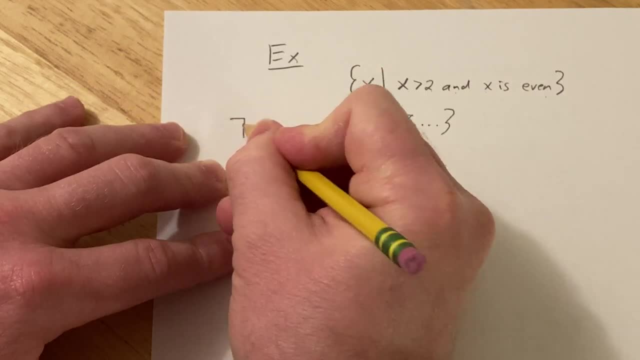 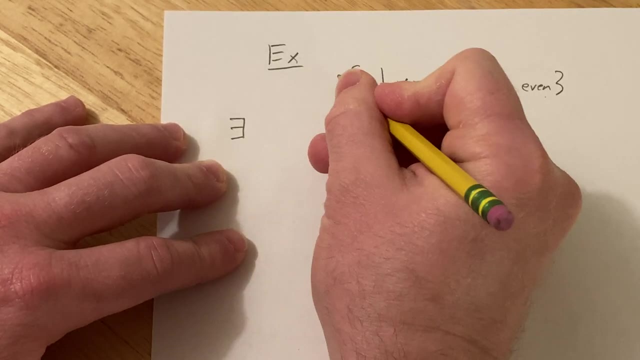 by 4.. So that's an example of how we can use this. So I can say: there exists a number in this set that is divisible by 4.. So I can say: let me give this set a name. I'll call it b. 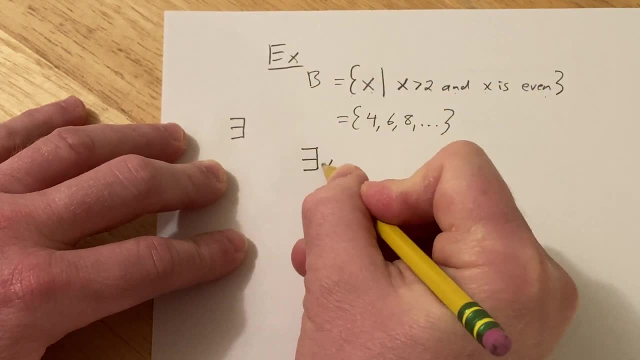 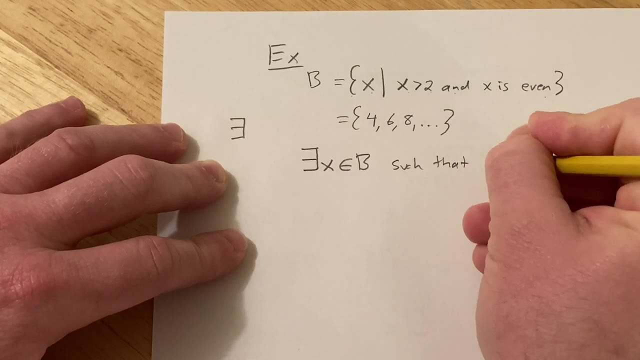 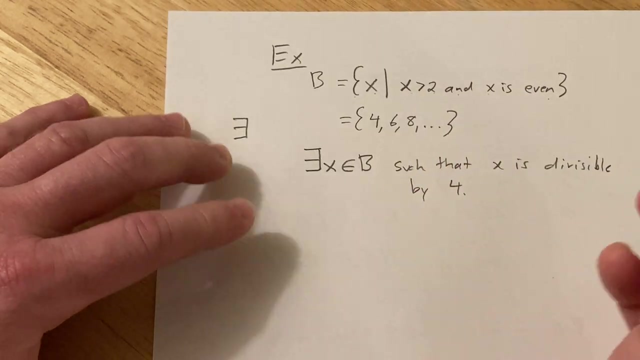 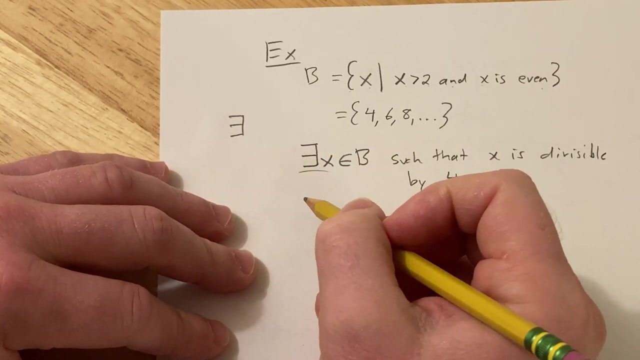 So now I can say: there exists x, x in b, such that x is divisible by 4.. So that's a simple example that I just made up right now on the spot of there exists. This is an example of how you could use this quantifier. 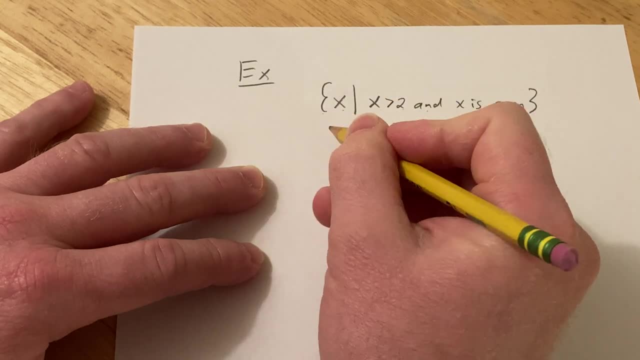 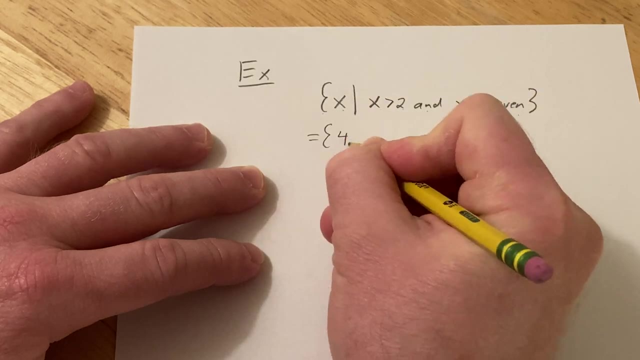 So this set has a bunch of numbers in it. For example, This is a set. This is a set. The first number that's bigger than 2 and is even is 4.. The next one would be 6.. The next one would be 8.. 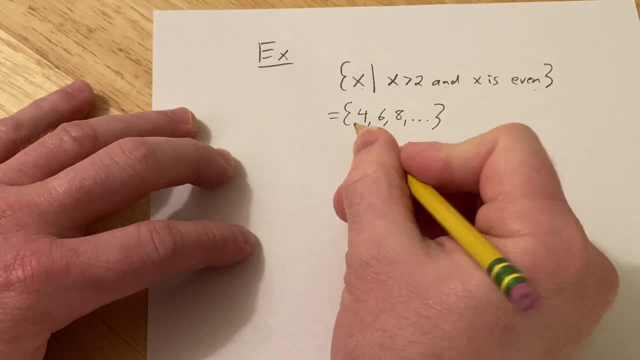 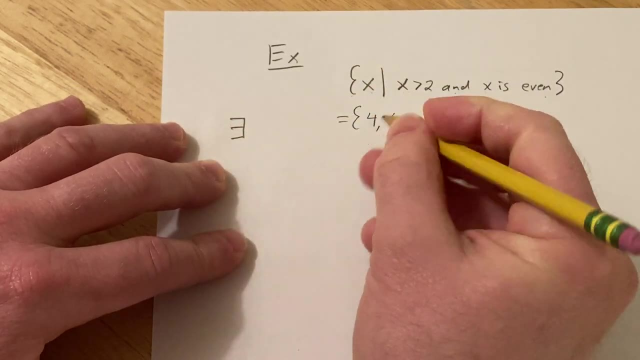 Etc. So what we can say about this set is that there are numbers in this set that are divisible by 4.. So that's an example of how we can use this. So I could say: there exists a number in this set that is divisible by 4.. 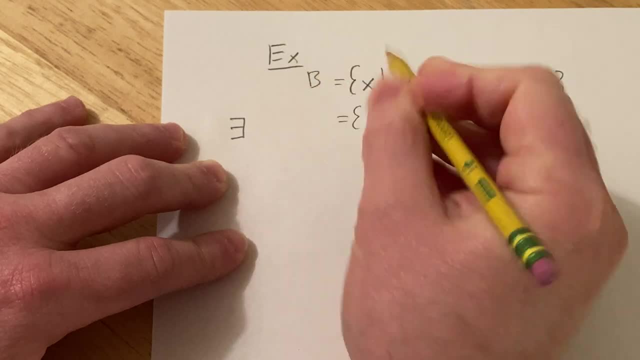 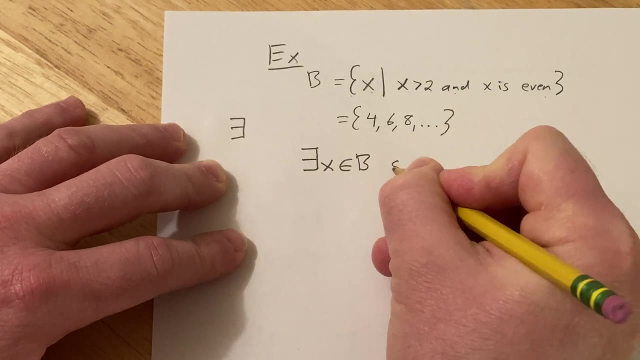 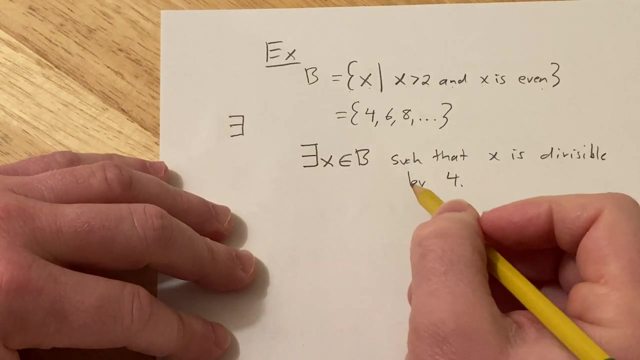 So I could say: let me give this set a name, I'll call it b. So now I can say: there exists x squared x in b, such that x is divisible by 4.. That's a simple example that I just made up right now on the spot. there exists. 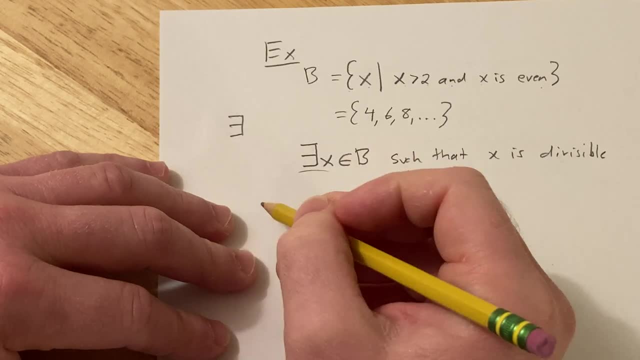 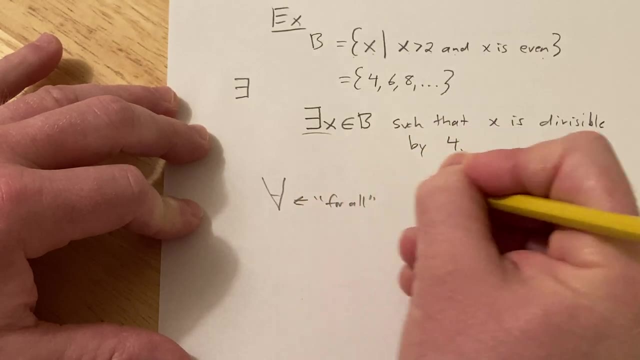 This is an example of how you could use this quantifier. So now you know two quantifiers. You know this one, This is the for all, And you know this one. This one means there exists. These come up a lot in calculus. 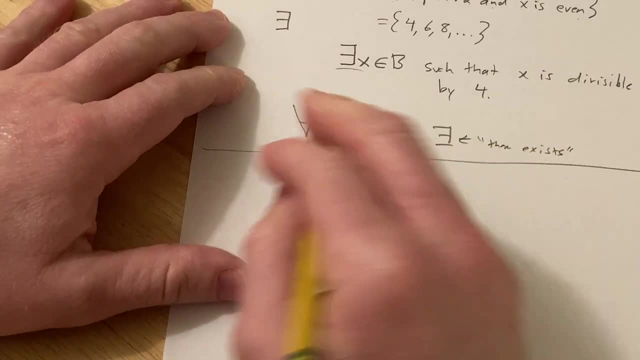 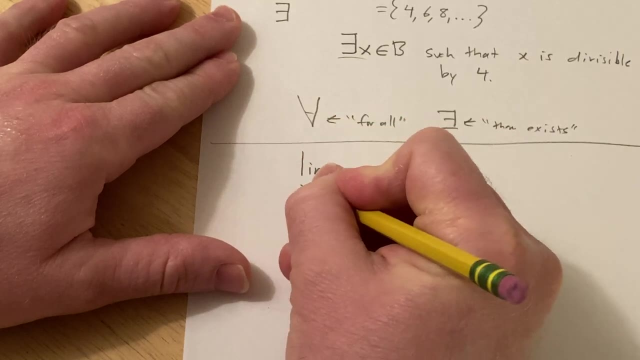 Let me give you an example, a hard example. Let's just go nuts, Let's just like unchange, whatever the word is. So in calculus you study limits. So you have the limit as x approaches a of f, of x equals l, where l here is a real number. 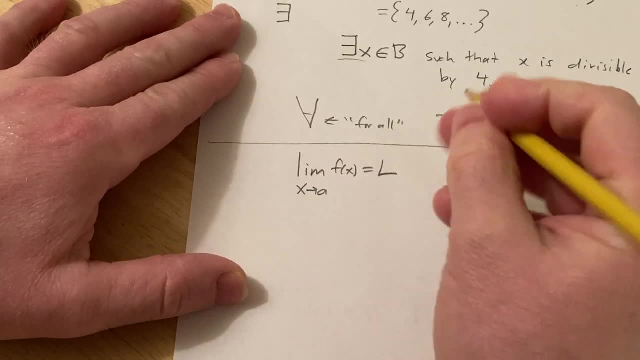 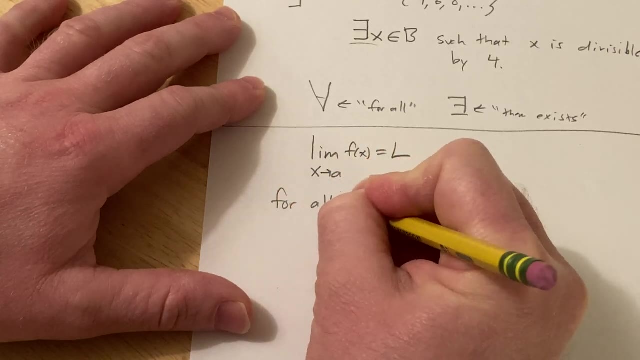 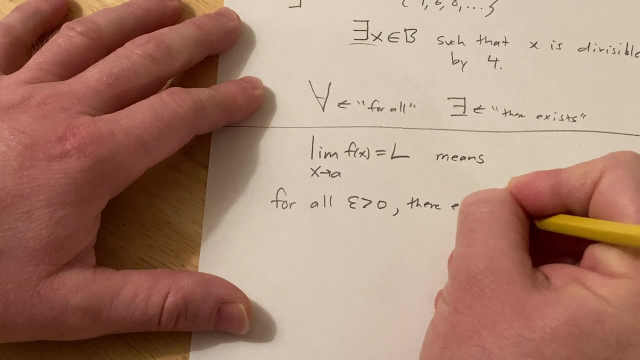 So let's assume in all of this, l is a real number. So what does this mean? This means? okay, this means for all epsilon greater than 0,. okay, this is what this means: there exists delta greater than 0.. 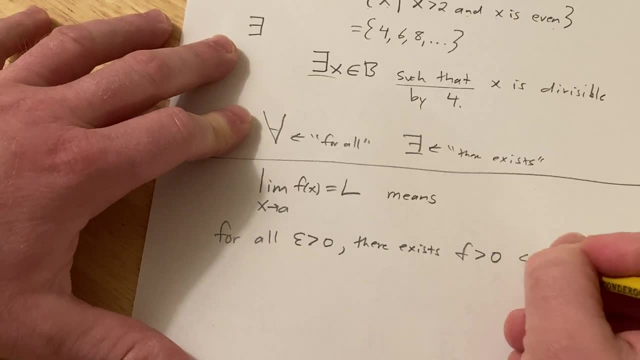 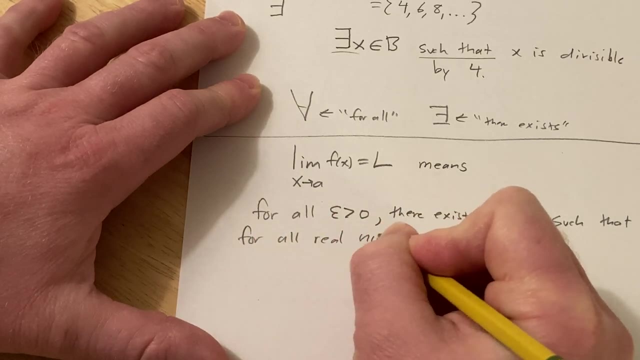 I'm going to abbreviate such that: with st, but I'll spell it such that: for all real numbers. So this is just the definition. So what I'm going to do here is I'm going to write the definition and then I'm going to write it using quantifiers. so you see how to use them. 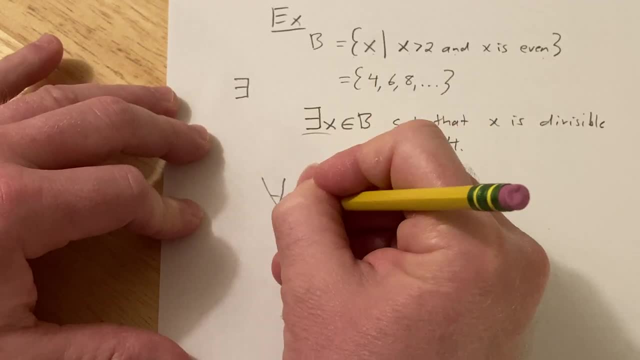 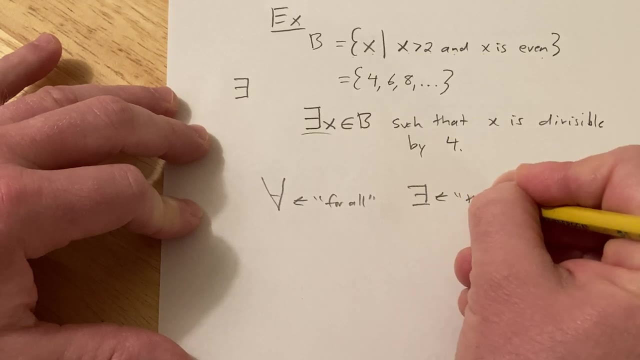 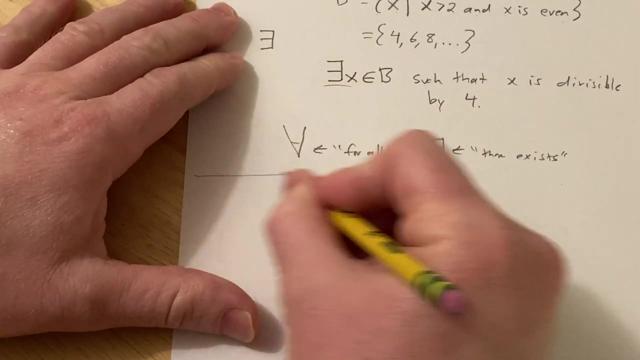 So now you know two quantifiers. You know this one, This is the for all, And You know this one, This one means there exists. These come up a lot in calculus. Let me give you an example, a hard example. 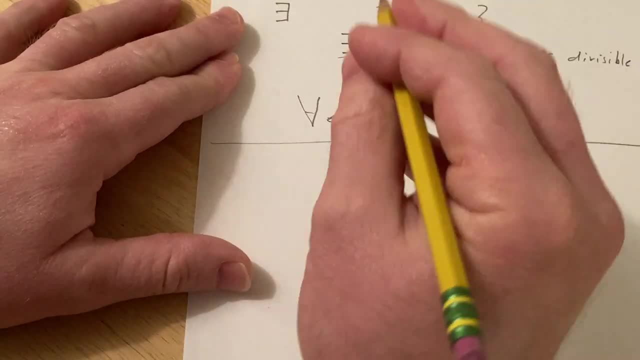 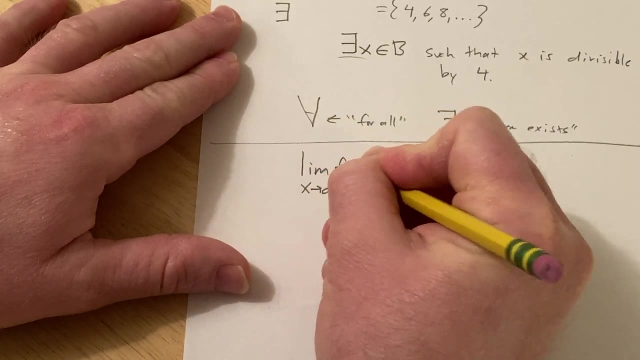 Let's just go nuts, Let's just like unchange or whatever the word is. So in calculus you study limits, So you have the limit as x approaches a of f of x equals l, where l here is a real number. So let's assume in all of this l is a real number. 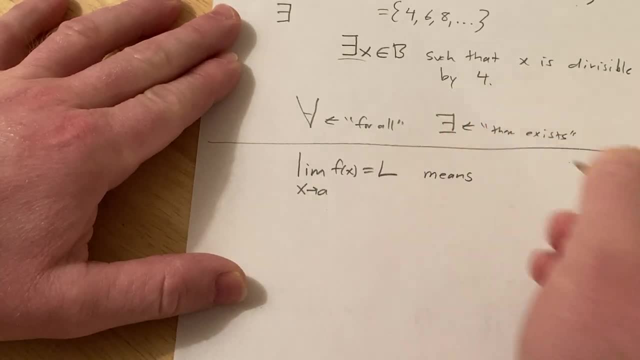 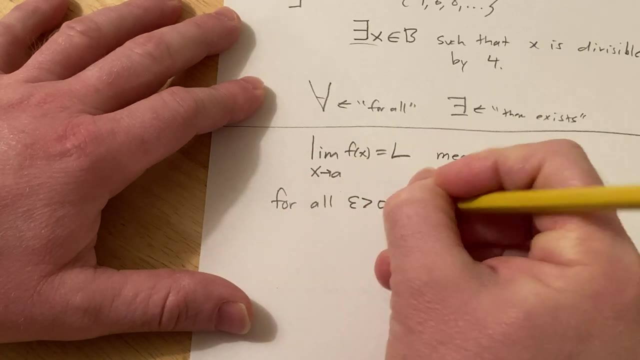 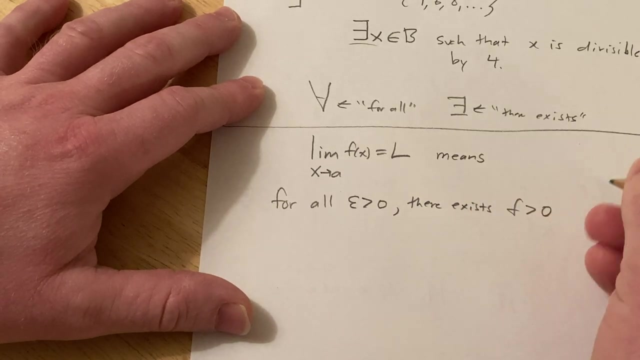 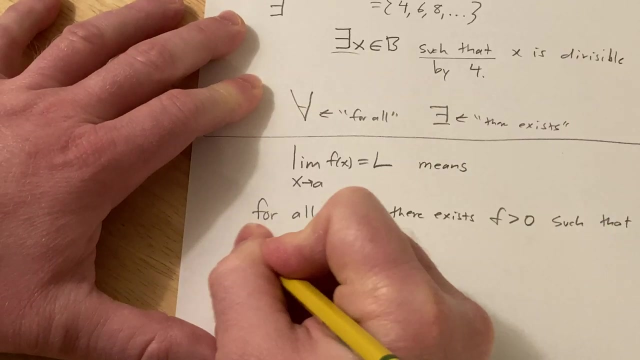 So what does this mean? This means? okay, this means: for all epsilon greater than zero. okay, this is what this means. there exists delta greater than zero. I'm going to abbreviate such that with st, but I'll spell it such that: for all real numbers. 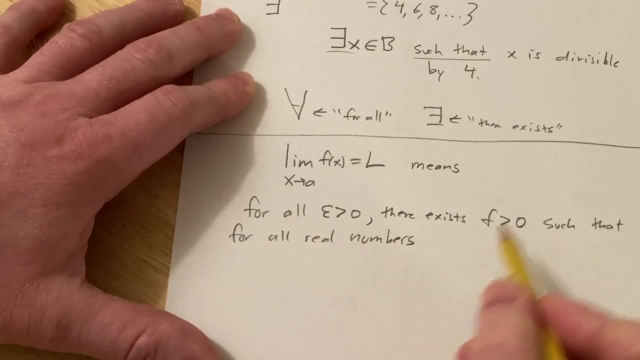 So this is just the definition. So what I'm going to do here is I'm going to write the definition and then I'm going to write it using quantifiers, so you see how to use them. So, for all epsilon greater than zero, 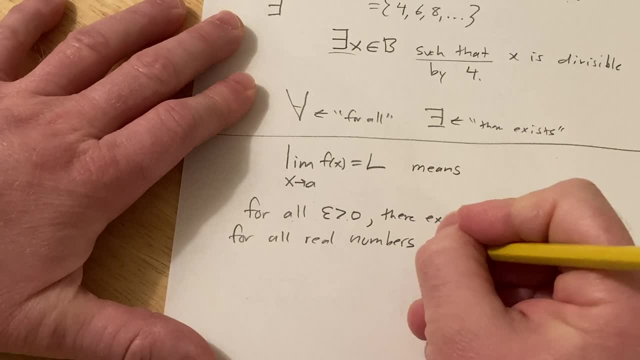 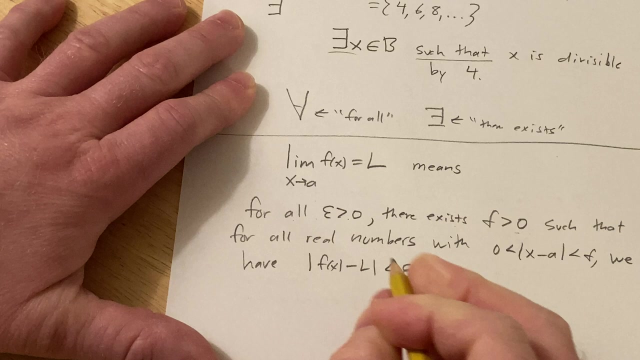 there exists a delta greater than zero, such that for all real numbers with the distance between x and a less than delta, we have the distance between f of x and l less than epsilon. All right, so now I'm going to take this statement and I'm going to write it using quantifiers. 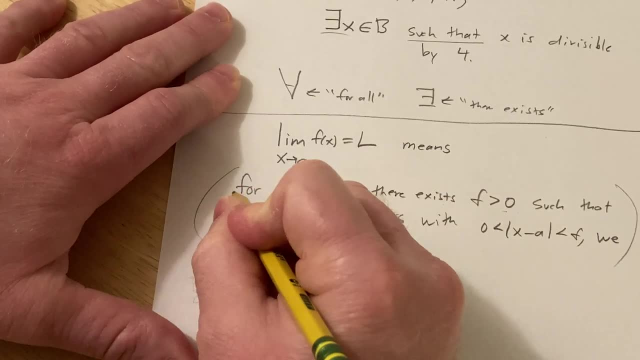 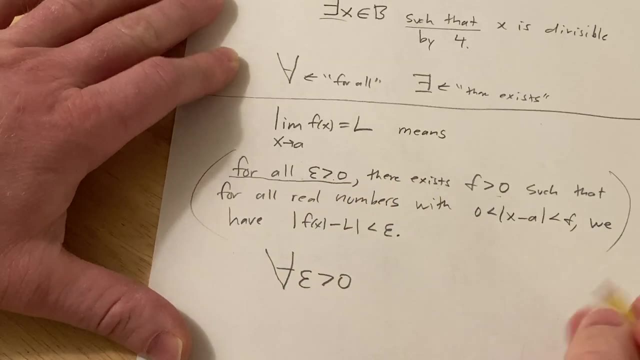 And hopefully you can hear me, This is very loud. There's a lot more outside. So, for all epsilon greater than zero, you can simply say: for all epsilon greater than zero, Boom, There exists a delta greater than zero. There exists a delta greater than zero. 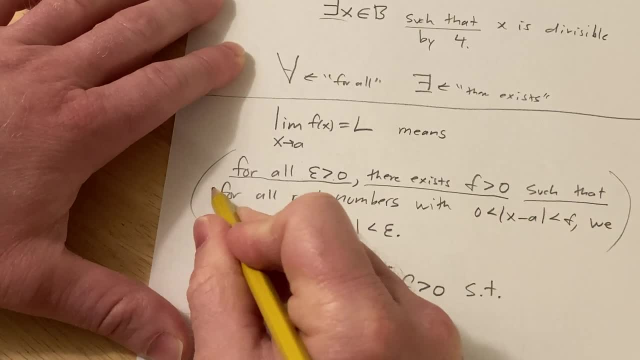 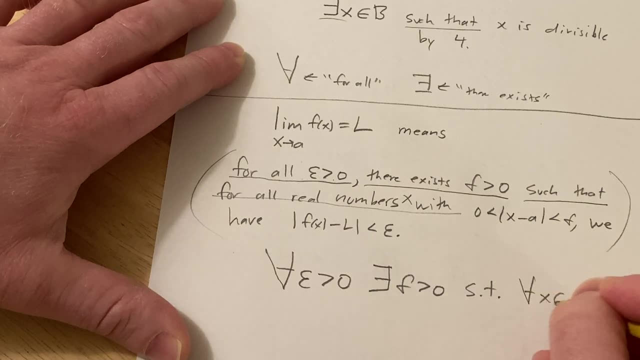 For, such that you can use st For all real numbers with, so I'm talking about the real numbers x. I probably should have an x here, such that for all x and r, with this inequality being true, we have. 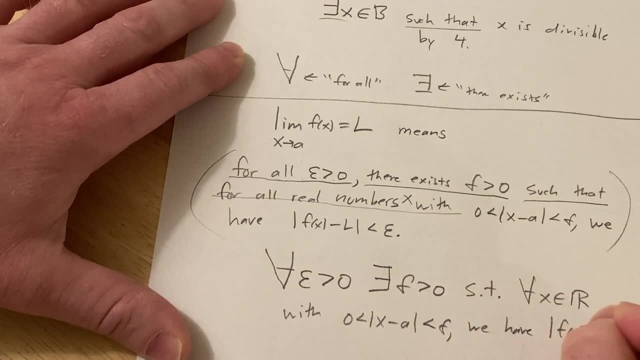 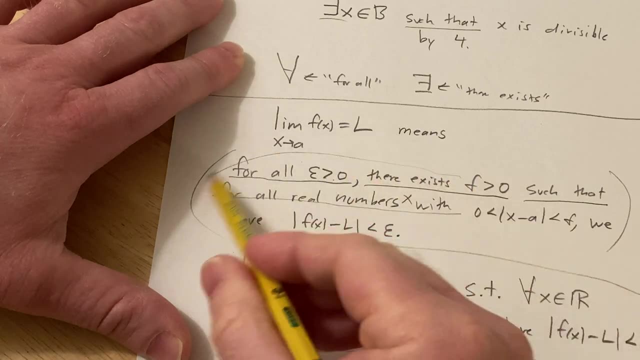 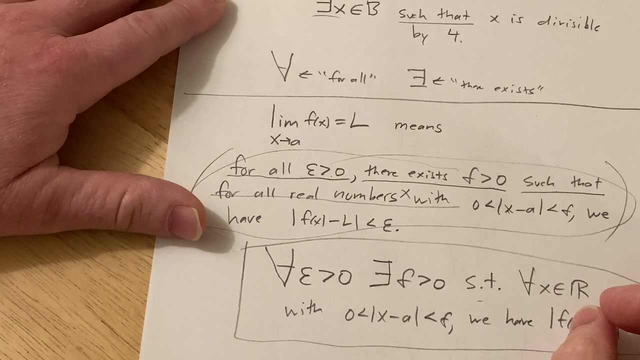 this, inequality being true. So that's how you would take the definition of a limit you would see in a calculus book perhaps, and translate it using quantifiers. So kind of a crash course using quantifiers. I went pretty quickly and hopefully you can hear me above the very loud lawnmower outside. 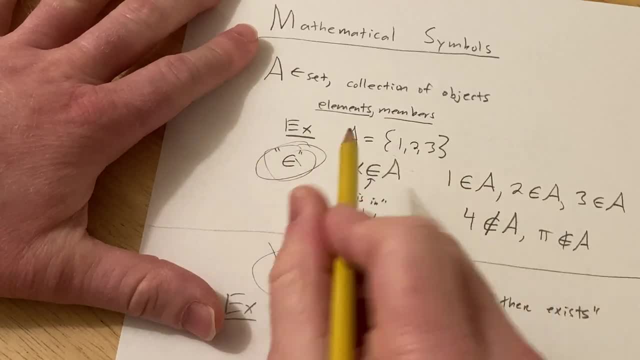 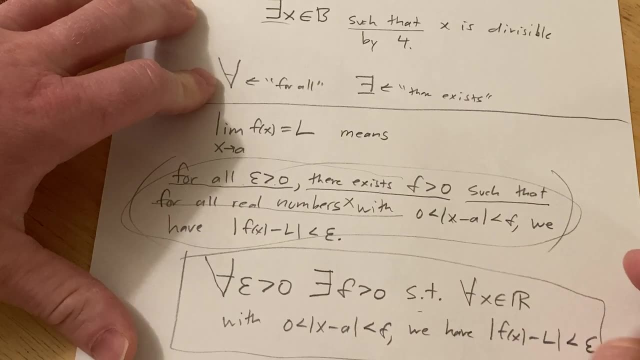 So yeah, So this one is belongs to, is in, is a member of, This is for all and this is there, exists. So yeah, just some extra life knowledge, Good luck. 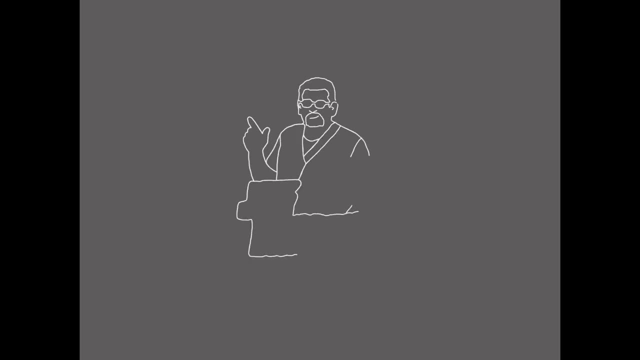 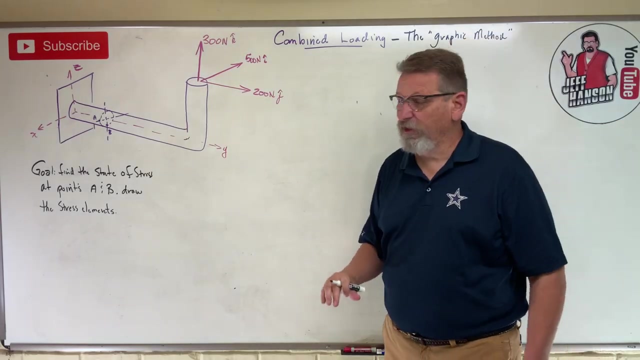 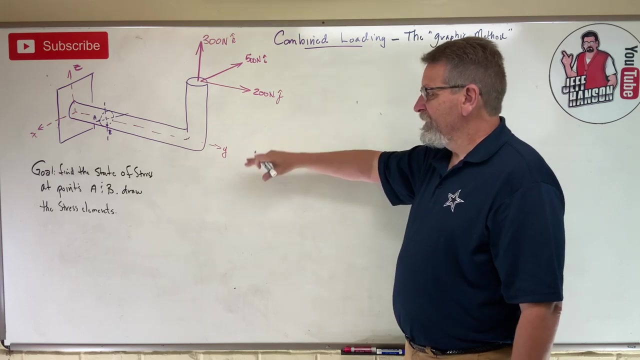 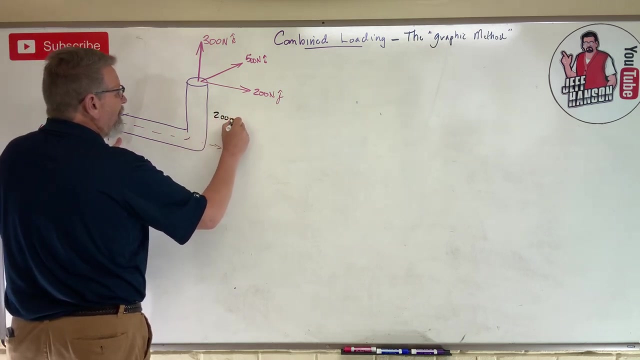 Hey gang, welcome back to the channel. Today we're talking about combined loading in solids. right, This problem is really stressful. We're going to find the state of stress at points A and B on this cross section over here, Let's make this 200 millimeters. 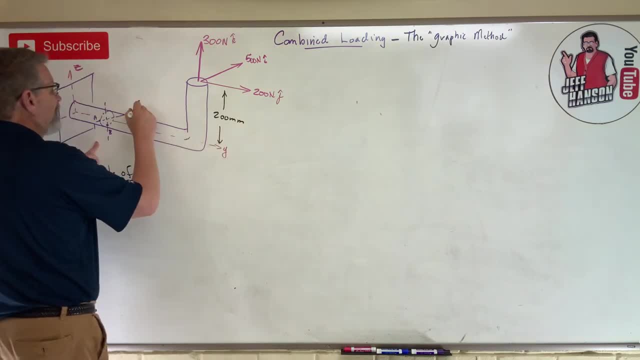 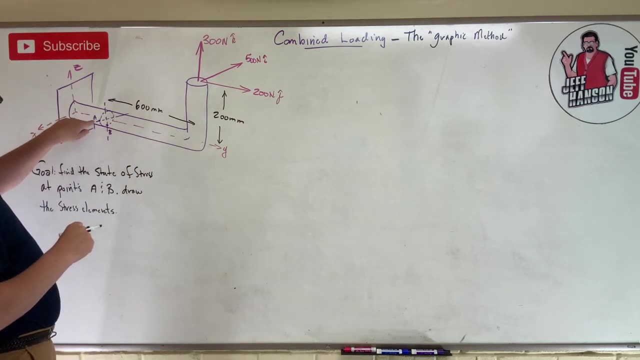 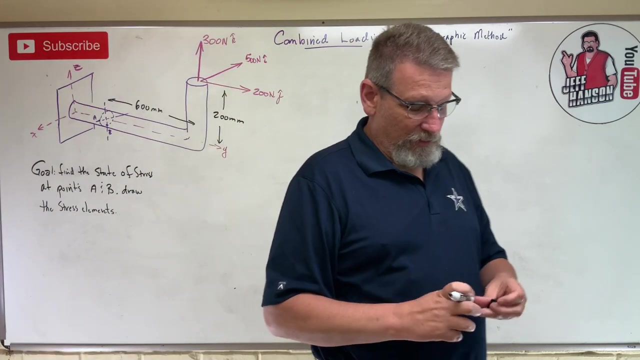 and we'll make this 600 millimeters just for funsies from there to there, okay. So the state of stress is at point A and point B on this cross section, okay, And they also want us to draw the stress elements, okay. So I know that this is kind of a tricky thing for you guys. 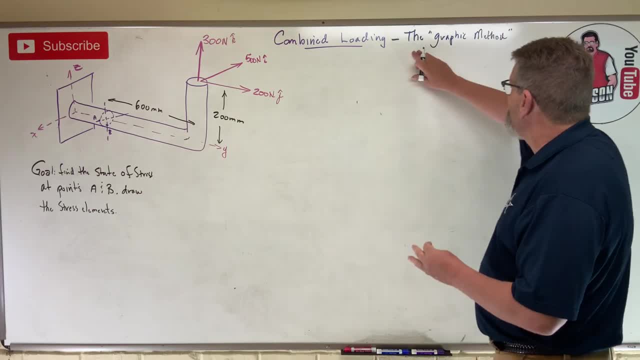 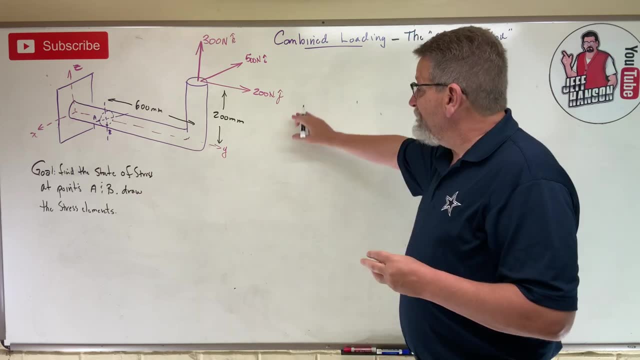 and so maybe this will help. Now I've got here, I'll call this the graphic method. okay, I'm going to show you a little bit different method. This is the way my brain thinks about this. A lot of people would have you write the forces in the x, the forces in the y, the moments around. 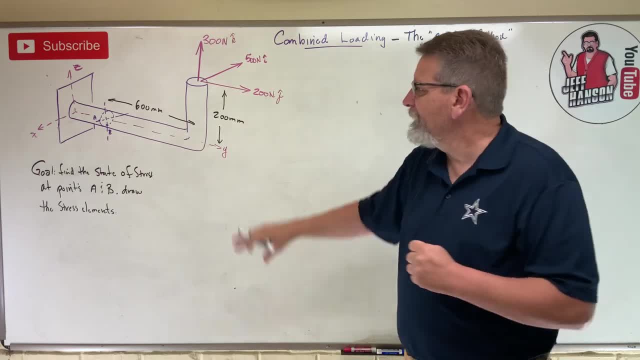 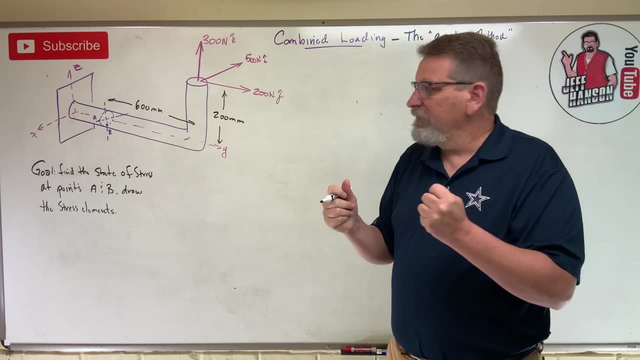 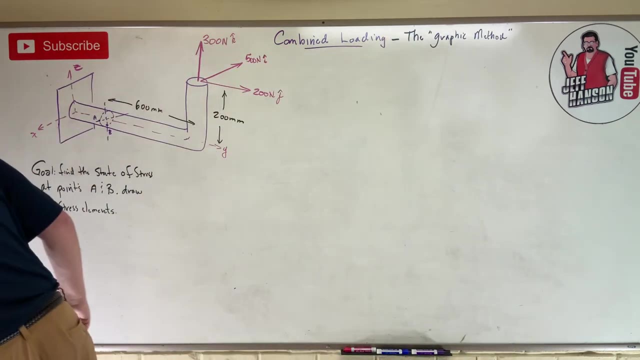 the x-axis, the moments around the z-axis, the moment around the y-axis, right, But you don't get a real understanding of what those moments, about those axes, really mean. You can't like see it, and I hope that this method will help you. okay, Now, here you go. One of the main things. 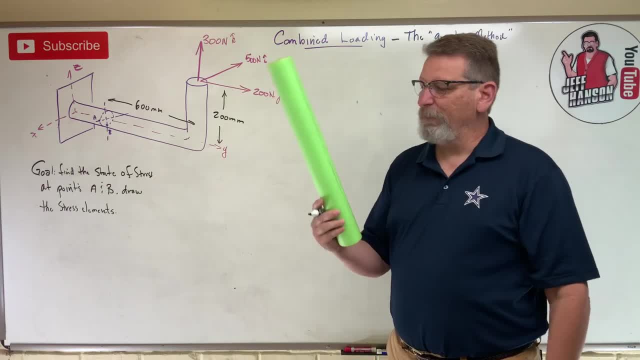 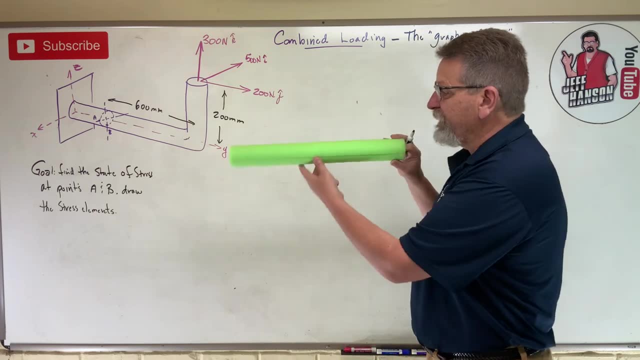 that's going to help you is this really helps if you have a little noodle, a little, it doesn't have to be this long, it can be this long, whatever right, And draw a line. see, I have a line drawn down here, right, So I can visualize if I'm point A and